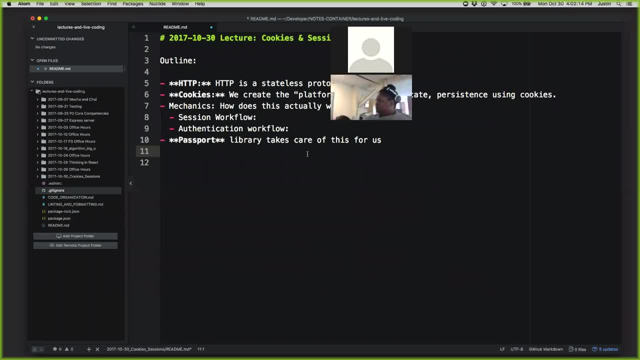 Sense of what the pace is, how the pace is going. So we're gonna talk about HTTP, we'll talk about cookies, we'll talk about some of the mechanics of how things are working, including how sessions work and how authentication works. 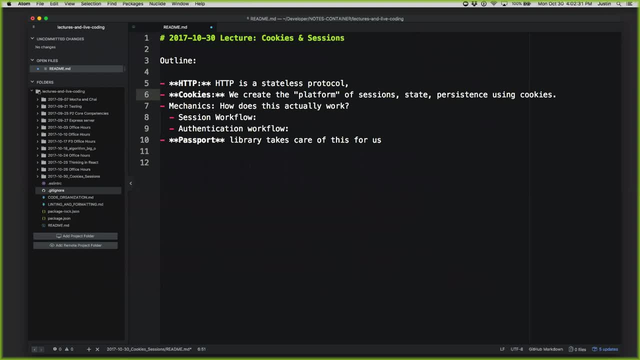 We'll talk just a little bit about Passport- the library that does a lot of this for us- And we'll have time for questions and curiosities. So HTTP is a stateless protocol- We're all aware of this And that has some very cool design features to it. 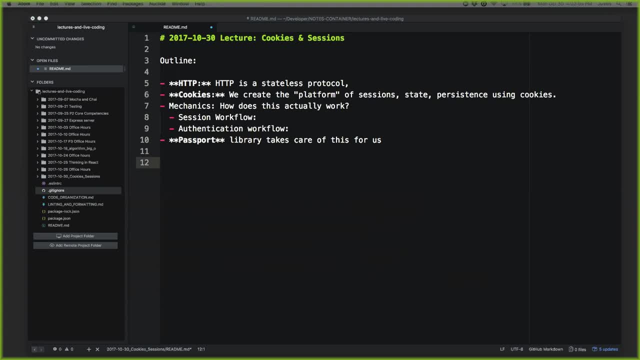 It also has the effect of making it not natively implementable To have continuity in your interactions with something that you're serving over HTTP. So websites, just by the HTTP protocol, cannot create the experience of like I log in on one page and I go to another page. 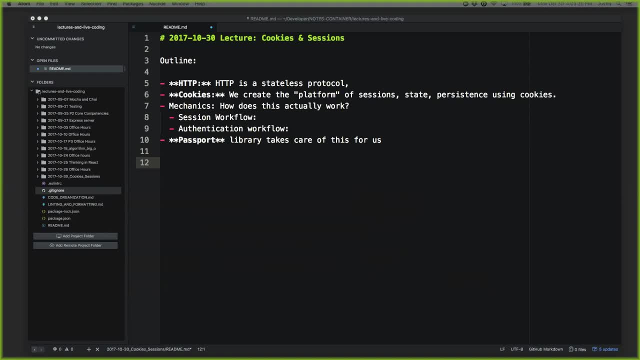 Or I add something to my shopping cart and then I go to the shopping cart and then there's the thing To do, that we need cookies And that's this, like now, kind of ancient browser technology that we've- we've co-opted for the purpose. 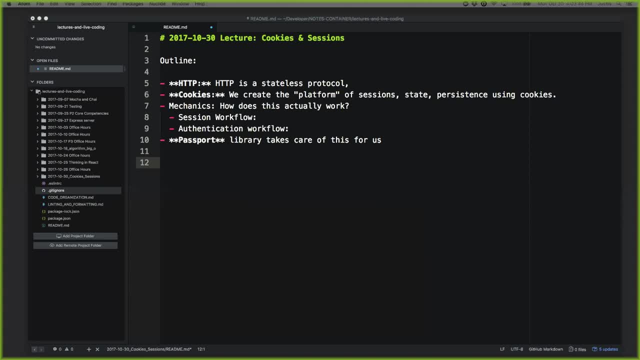 of creating this ongoing thing that we call sessions, Right, So let me back up for a second. So, HTTP in HTTP, every request is handled independently. Even though it seems like there's continuity between it, Each request is considered by the server in isolation. 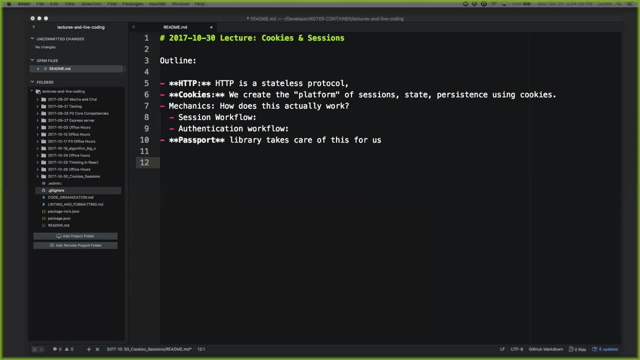 But again, because state is necessary for basically any web application we have, we use something built on top of HTTP, which is this cookies and sessions thing. Cookies are the vehicle for creating sessions, You know. you can think of it sort of like the. 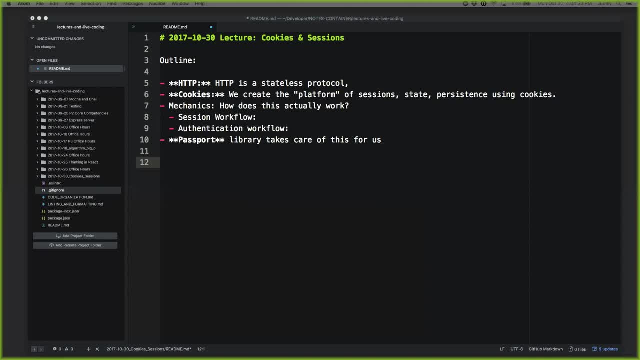 having like a hello, my name is sticker. That like if you were at a party where nobody was remembering anybody's names but you had this sticker, then you could go up and talk to someone and you could initiate a conversation. They'd be like: oh hey, Eugene, it's great to see you. 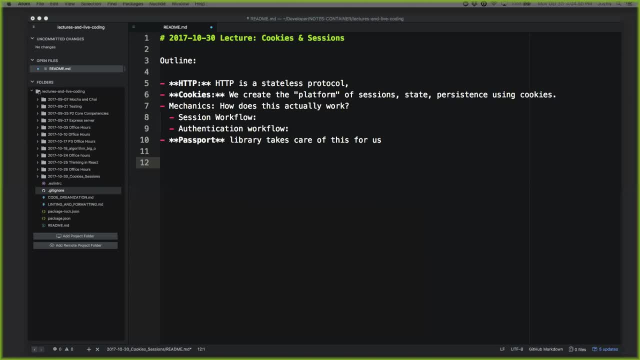 And then, if they forgot your name, they'd come back and oh hey, Eugene, it's great to see you, Because every time you're, they're seeing this name tag that says this is who I am, And so that's what cookies help us accomplish. 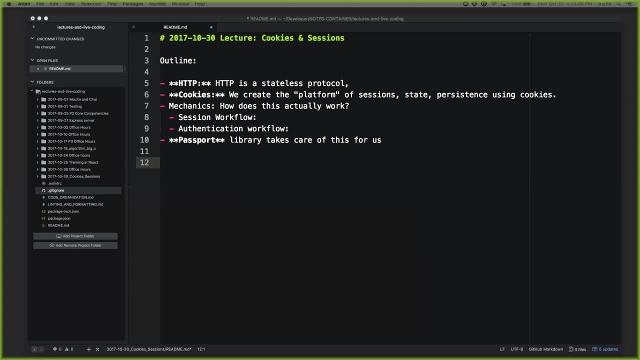 We know about how cookies are implemented, That cookies are sent in a response, HTTP response, and browsers manage the like, acceptance and storage and deletion of cookies right. So if you send a request to googlecom, Google is gonna send you back a response. 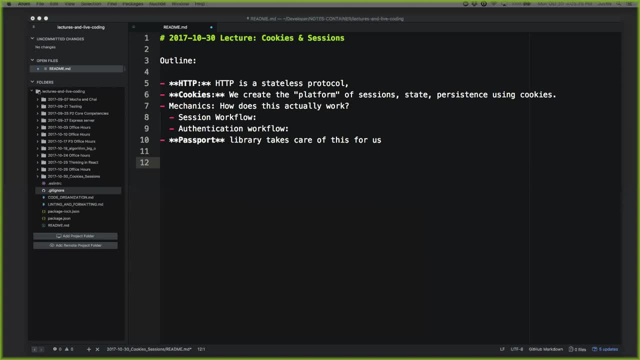 And in that response it's gonna say: oh, by the way, please set X and Y and Z cookies, And actually it's probably like A, B, C, D, E, F, G, H, I, J, K. 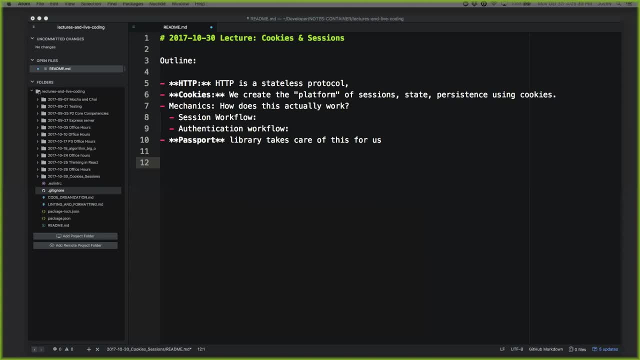 and Z cookies, because we use cookies for everything really. So it's all managed by the browser and the server, but not actually through the HTTP protocol. That's one thing I just want to kind of make sure we're clear on. is that like it's this thing that we use? 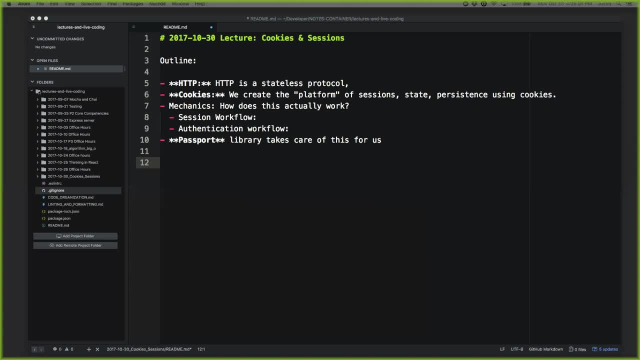 on top of HTTP, And so the browser is the thing that knows how to read that header that says okay, That says here's a cookie, Here's its name, Here's the value, and Then it knows to send that again with any subsequent requests. That's that it makes to that same domain. 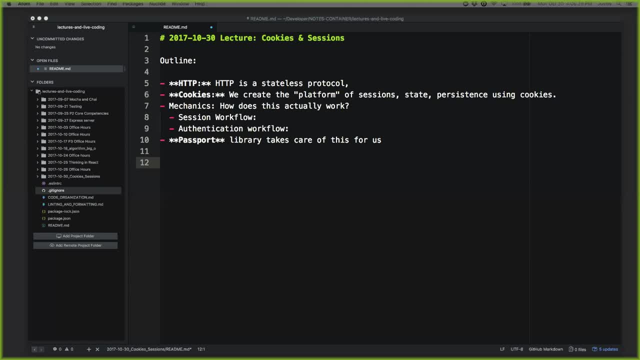 So, Yeah, any questions so far. So with session. yeah, That's more of a slight clarification. when you say cookies, and I guess the ultimate question is are, Is it one of those who has always required us and sort of middleware or What do you mean middleware Asking, if cookies are? 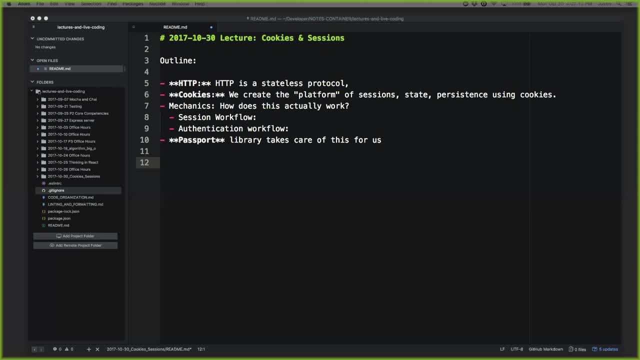 Are they more part of the warehouse or are they more part of what I guess powers HTT? It's a good question. so Cookies are it's kind of like. what do cookies belong to? Yeah, Yeah, That's. that's kind of the funny thing, because cookies are just a header among. 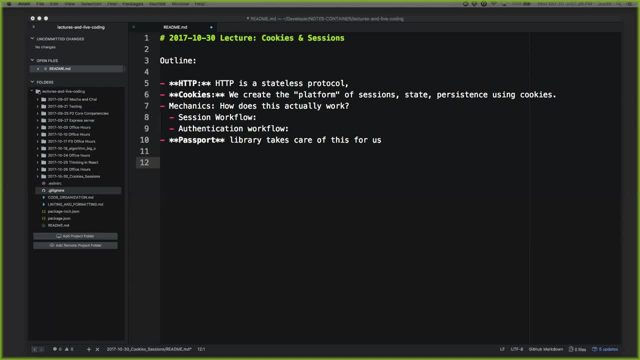 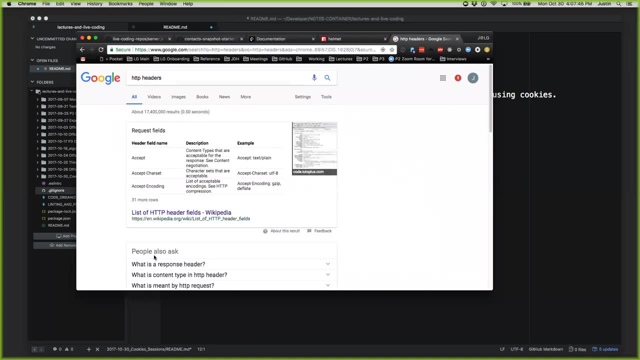 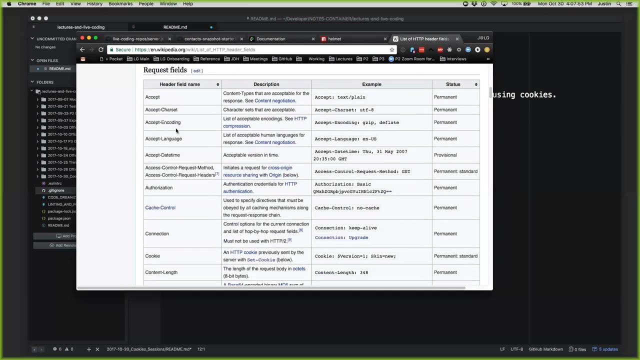 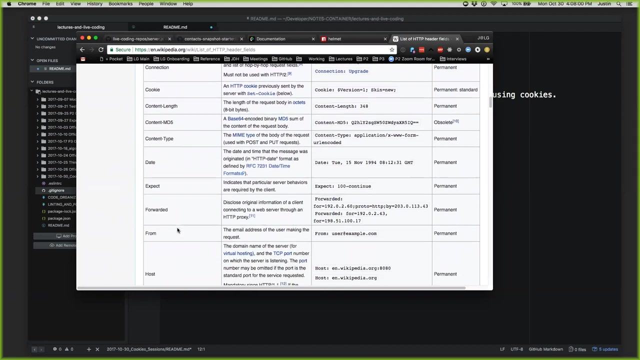 All sorts of other headers. right, HTTP has a bunch of different headers. You can see There are bajillions of them. What do I accept? accept encoding, cache control, There's cookie Content-length, you know all sorts of things. so it's to to HTTP. It's just another header, That's that's. 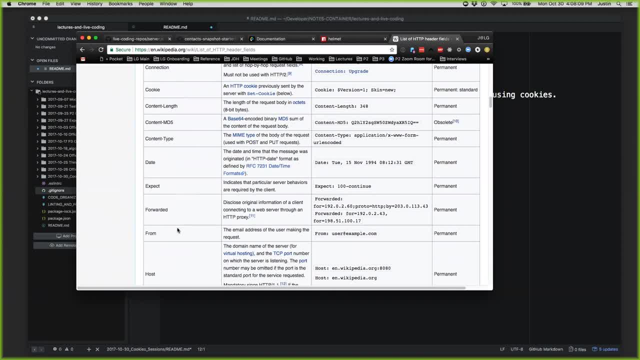 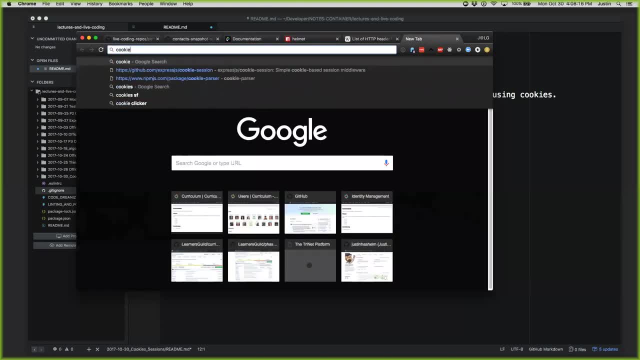 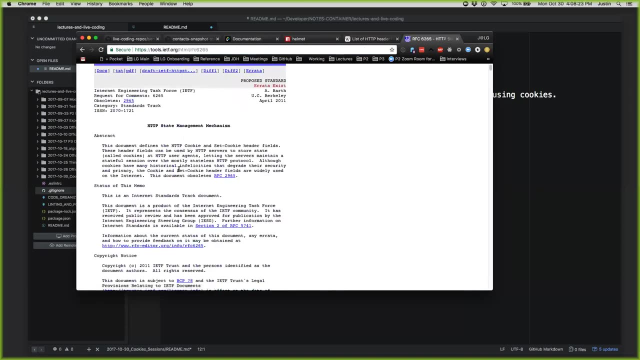 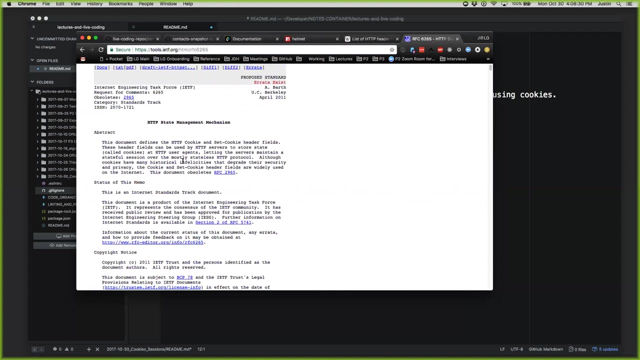 what I'm meaning in terms of, like, it's built on top of HTTP. I bet cookies are actually standardized. Yeah, I'm wondering So. yeah, So do you guys know what RFCs are? So this is like the, the way that internet standards are created. 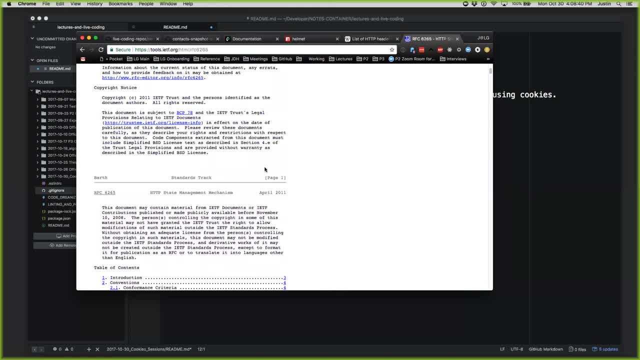 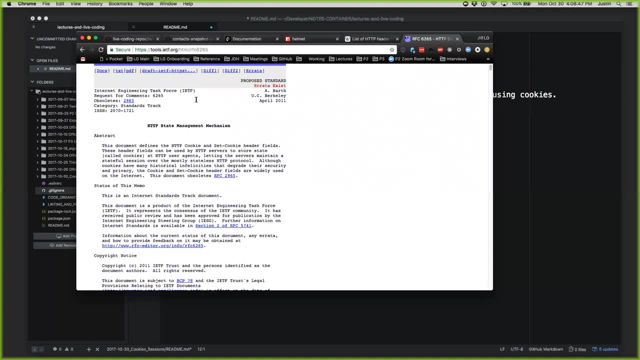 And I think it stands for request for comment, And so this internet engineering task force. they come up with a proposal that put out a request for comment and some things get accepted, And so, like: HTTP is an accepted spec as defined by RFC, whatever, whatever, whatever. And when you send email, 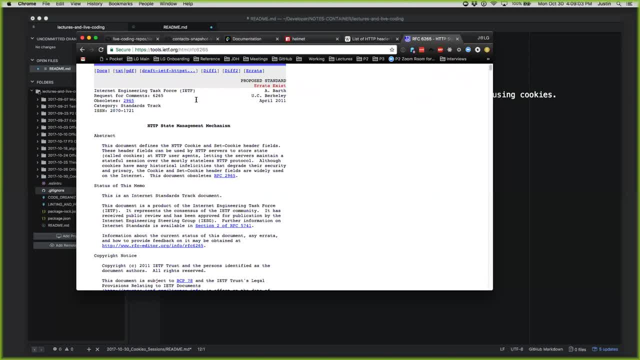 like the protocol that you use to send email, SMTP and the headers that are sent and everything. those are also standardized through an RFC. Notably REST, and what it means to be RESTful is not standardized in an RFC, And I think there was. 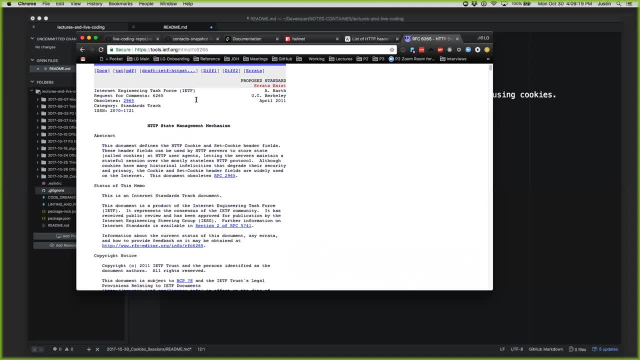 an attempt at one point to do that And, for whatever reason, they decided not to make it like an official standard, which is part of the reason you'll hear us talking about it as like a set of kind of guidelines, and people implement it a little bit differently. 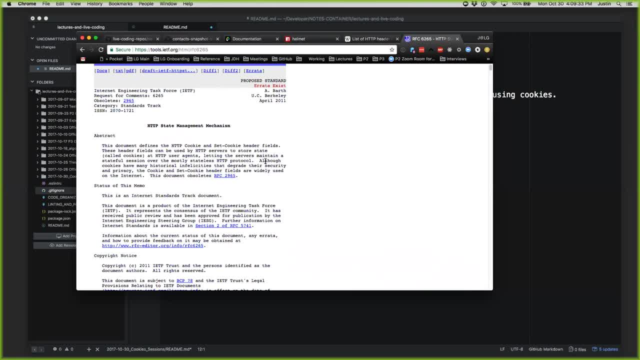 Where was I going with this? Cookies, What they belonged to As in being a header. Yeah, that's what we answered. Yeah, and I mean it's they kind of belong to this like mutual agreement or the standard between browsers and. 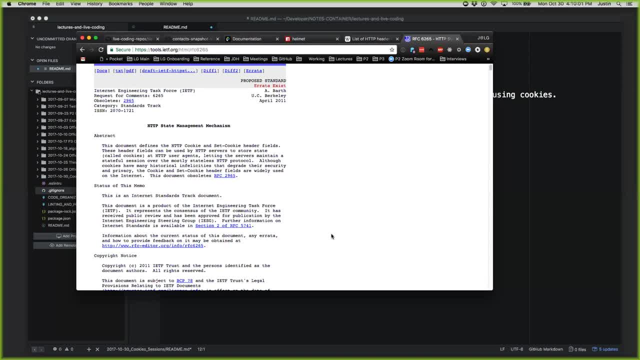 servers right. So servers set cookies, browsers are implemented to receive cookies and work with them And it's like that's the kind of place that cookies actually live is like in this mutual agreement between servers and browsers. Servers say: I'm going to send you some cookies, You don't need to know. 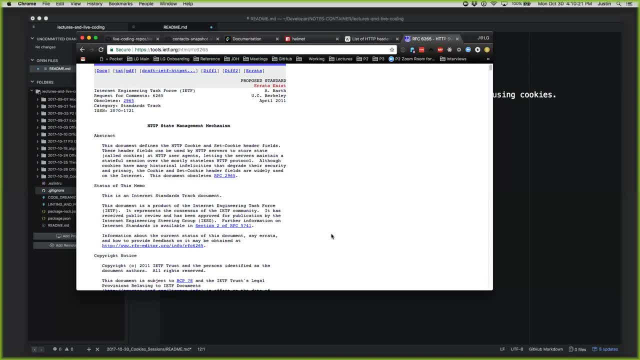 what they are. You don't need to know what they do, You just need to send them back next time you make a request. That way I can create continuity in your experience and also track your Internet. you know stuff and do analytics and all the other things that cookies do. 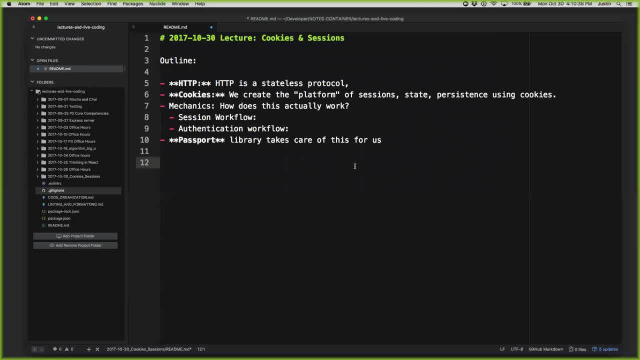 But, yeah, it's a good question: Where do cookies live? Yeah, so sessions, then, are the experience of continuity that we implement on top of cookies. So if you've done the authorization snapshot, you know that Express has, or the node world has, at. 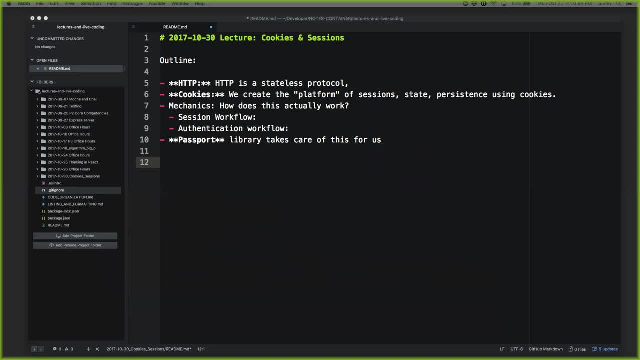 least two good cookie libraries. One is cookie session, one is Express session. Do you folks know the difference between the two? Like one of the main differences: One thing from the client side and the other thing from the server? good, Yeah, that's right. A cookie session puts the session data in. 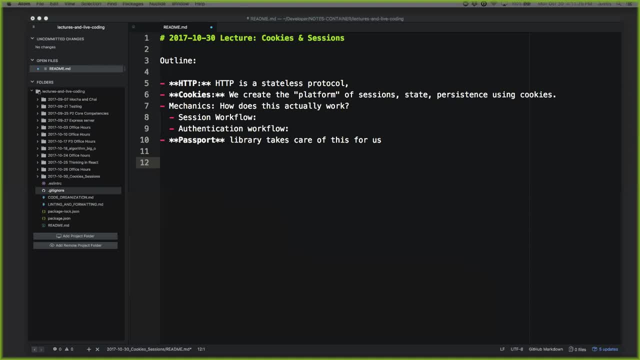 the actual cookie and sends that over with the HTTP response, right? So if you put some things in the session like a username and a role to the horseradish, they can add an teamed invite, Okay. But once they ask you to send code, they don't give you the oder andIGH, and even so they don't. 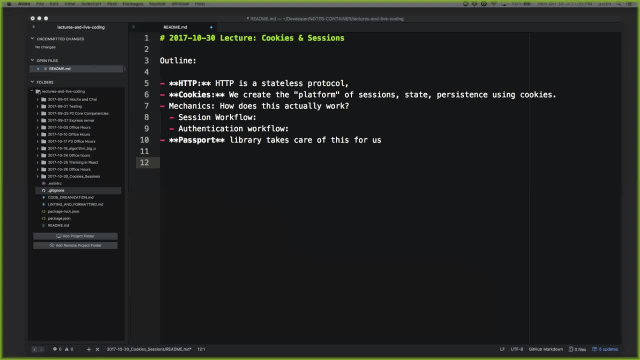 have to send it back. All you have to do is pop in a class and send them application student and whatever else. it will actually send that over to the client and keep that data there, versus Express Session, which tracks all of the session information in a store of its 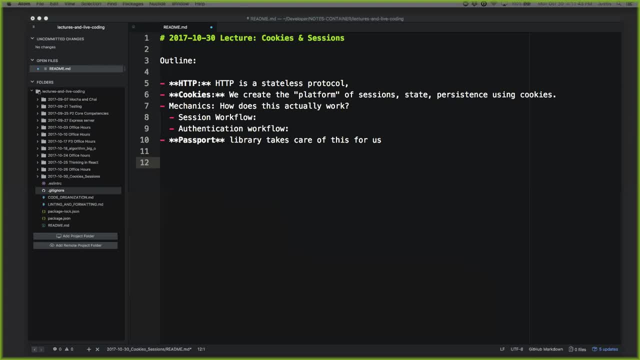 own and the default store for that is memory. You can also set it up to use PG Database. You can set it up to use something called Redis, which is something that's used a lot in production for storing session information like that in a way that doesn't fail when. 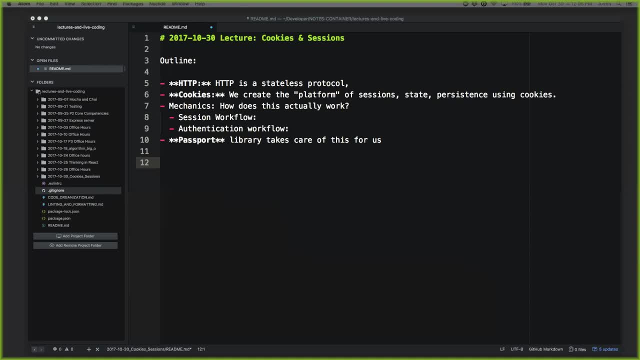 the server shuts down. So that's one thing you may have noticed. If you've created a session on some Express server and you're just using Express Session as built in, if NodeMon restarts that server, all of the sessions are wiped away, because 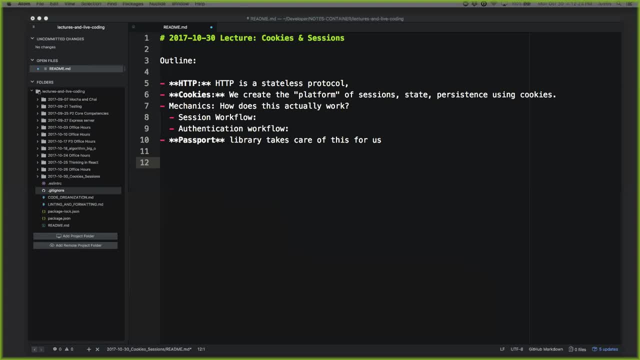 the sessions are Again by default stored in memory, and every time NodeMon runs, it actually just throws away the whole program and starts it over again, and so that's why we use something like Redis to maintain persistence of sessions. Yeah, so one important thing about this is that the data sent to the client needs to. 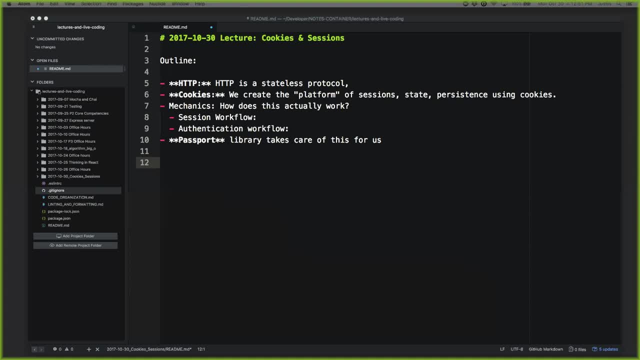 be encrypted. Why do you suppose that is That, whether it's a session ID, like with Express Session, Express Session is just sending a cookie with an encrypted session ID- or whether it's the actual session data- in the case of cookie session, why do you suppose it needs to be encrypted when it's sent over? 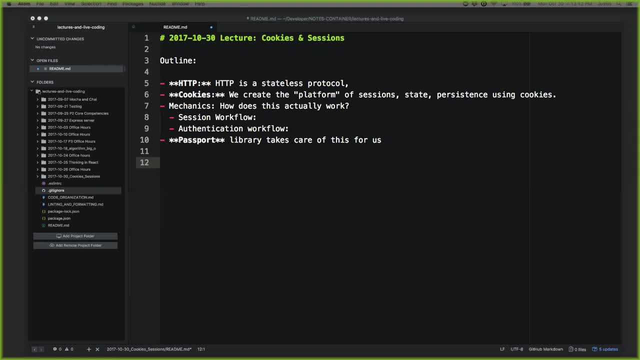 to the user. Okay, so that's one thing. It could be intercepted in the middle and we don't want. We don't want that to happen. We don't want people to be able to use it if they do. Okay. 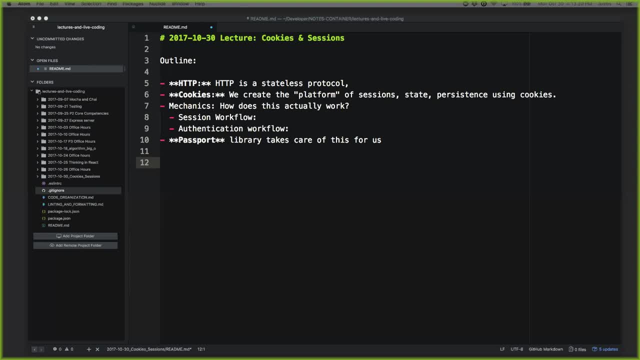 What else? I thought it was going to be like 100 or something like that. There's this kind of axiom in web development like there's front-end and back-end web development. There's this like axiom in web development which is like basically anything can happen. 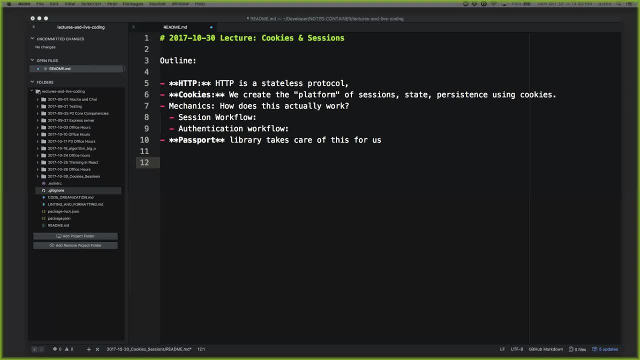 on the cloud. You don't want that to happen on the client side. You know you have client-side JavaScript that runs, but you don't have any idea if the client is going to run it correctly. You don't have any idea if the client like: if maybe there's a user on the client side. 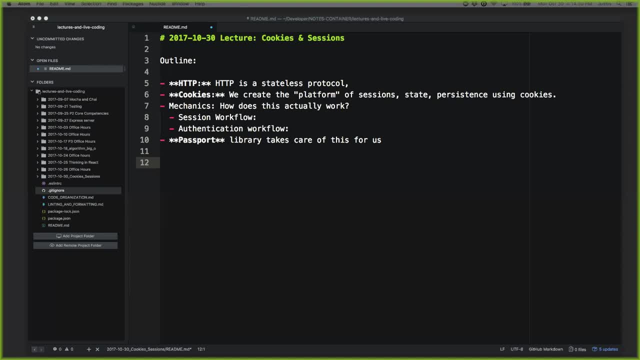 that's going to modify your JavaScript, because there's, Once you've sent it over to the client, if it's anything that's executing on the client side or exists on the client side, you have no control over how it's executed. So this was something they came up with. 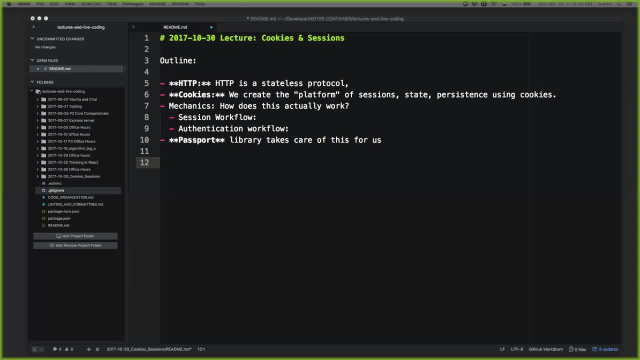 Bybov and Miles were talking about like implementing authentication flows in a front-end React framework. So right, React is something that's loaded and run entirely on the client side. But the problem is, if you implemented it just on that client side, just on the front-end, 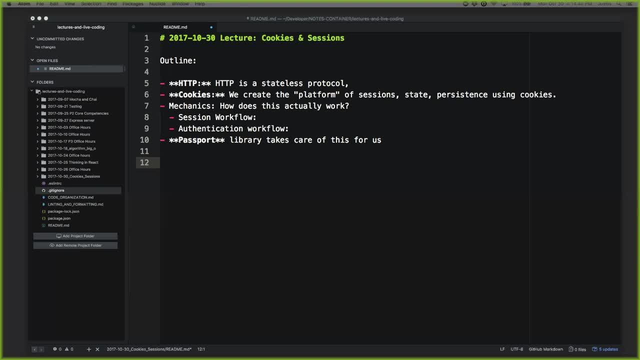 or just sorry, just on the client side. if you implemented authorization and like access restrictions and stuff just on the client side, there'd be no reason that the client user like you or me or anybody couldn't go into their Chrome dev tools and change. 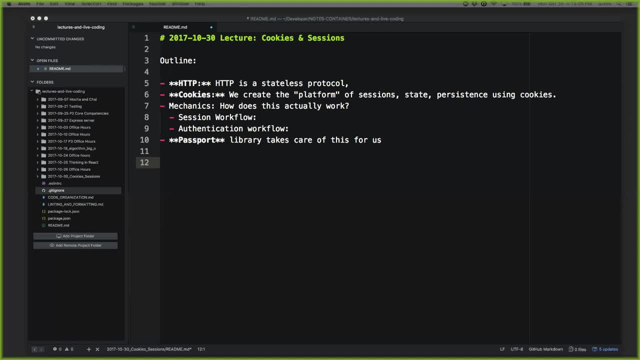 their user role, from user to admin And all of a sudden then they've got access to everything. So there's this thing to keep in mind, which is like we can do some pretty amazing stuff on the client side now in terms of these front-end frameworks and everything that we've done. 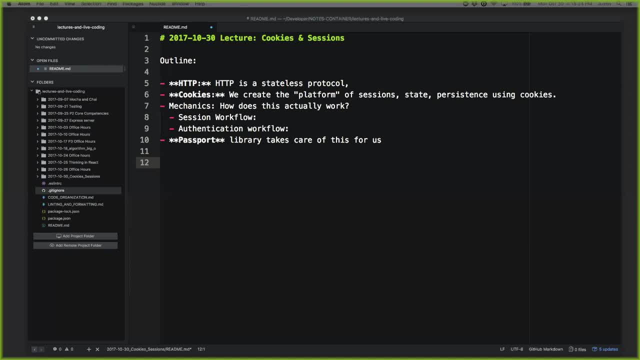 Everything that we can accomplish with that, But anything can happen over there, And so it wouldn't necessarily be necessary to encrypt a cookie if you were sending it over to a user that you trusted totally and completely. But if you don't like- for example, if we're using cookie session and we don't totally- 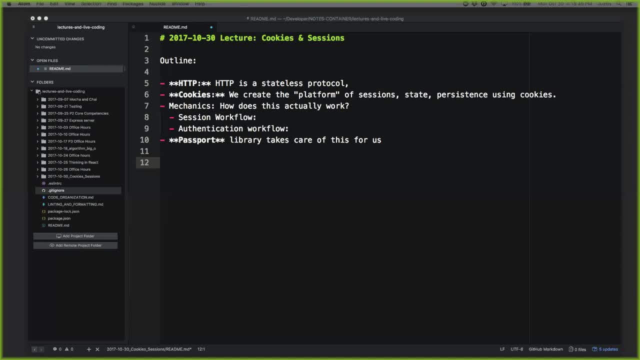 trust our users, which is a good position to take. If we sent over a session information that included I'm user X and my admin privileges are like true or I have admin privileges, Or say we said that we had user privileges, that person could go into that cookie and 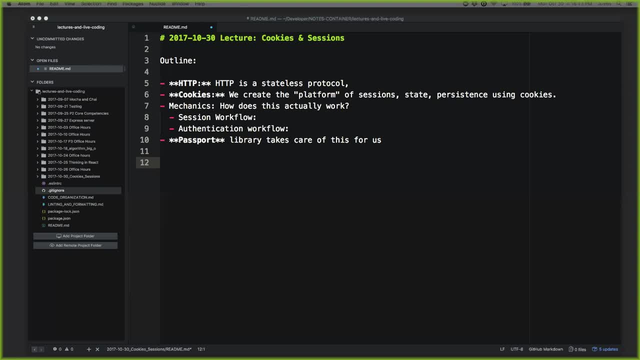 just change it and all of a sudden have admin privileges. So we don't want them to be able to change the cookie, And so that's one of the main reasons that we We don't want them to be encrypted, right? Just to kind of note that it's useful also in programmatic APIs, so like REST APIs. 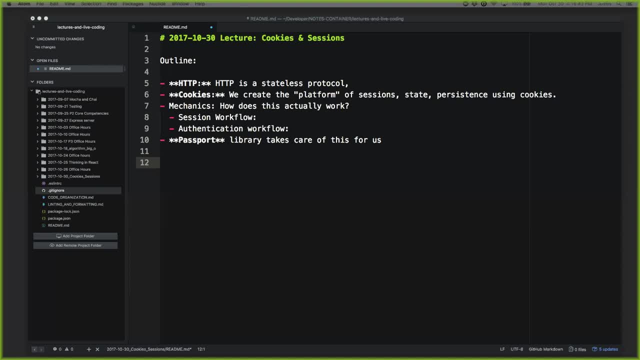 It's useful to have the same experience or to be able to create a session, namely, like you have someone accessing your data, You want to be able to authenticate that. You want to be able to authenticate them and then allow them to access certain data. 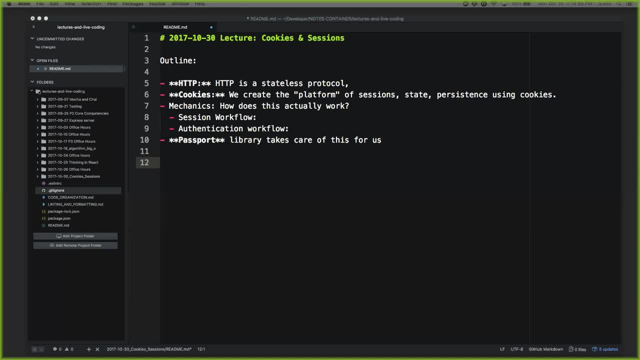 that they would only be able to access if they were correctly authenticated, And so it's the same principle at play about wanting to create like a session so that a person can continue to access protected data, But when you're talking about APIs and accessing them programmatically, you no longer have. 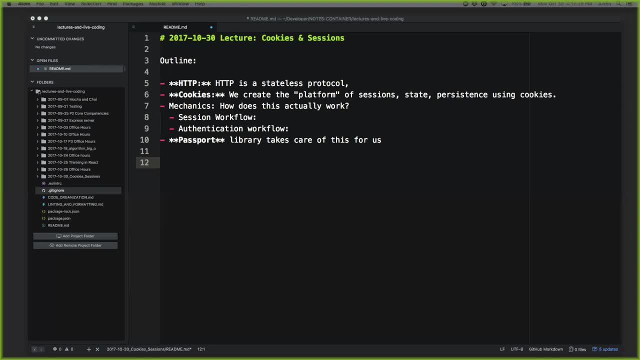 a browser in the mix. So it no longer makes sense to work with cookies And, in particular, what does make sense, or what usually is used, is some kind of token that you, the user, the client, through their API, logs in and then they receive a token. 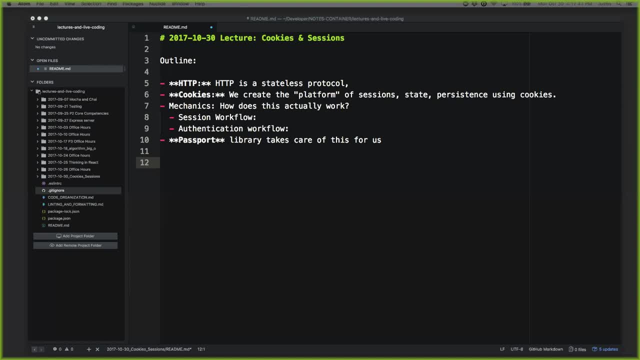 and they just send that token with every request. So it's the same idea as a cookie that you're sending this cookie with every request, But instead it's like some sort of token string that you can put in the headers. If you're doing GitHub, this would be the way that you could not just read some information. 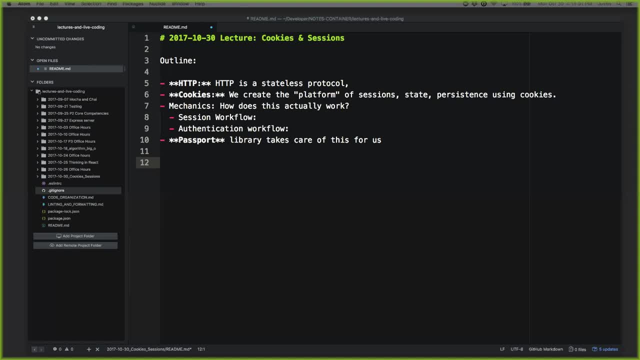 from GitHub but go to a particular repository and you could add a star and you could make all sorts of edit and delete operations because you had been authenticated. Cool, Any questions so far? Is this useful? Yeah, Cool, Okay, Yeah, so the kind of mechanics. how does this actually happen? 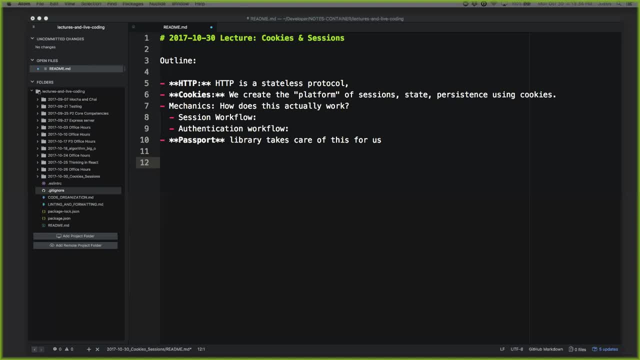 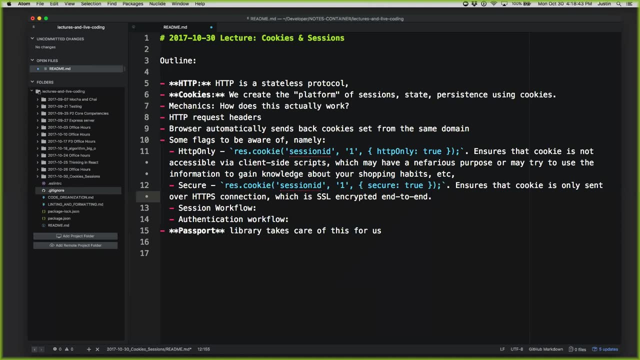 What's the back and forth? I'm going to actually just copy this. copy my notes for this. So It happens, through the HTTP request headers, browser gets sent cookies, it automatically sends them back. There are a couple flags to be aware of with cookies. 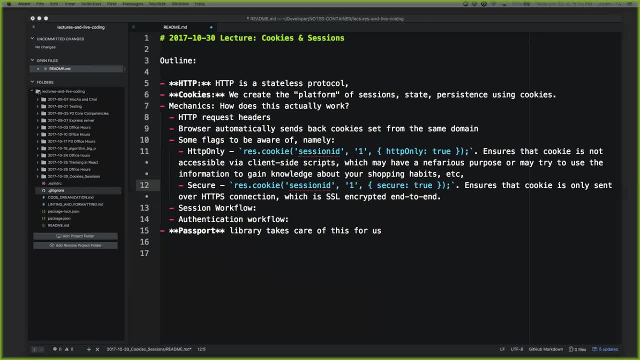 So this is in. I'm trying to remember if this is built into Express or if this is part of a particular library. I think this is built into Express. Yeah, So cookies can have these particular flags. One of them is HTTP only. 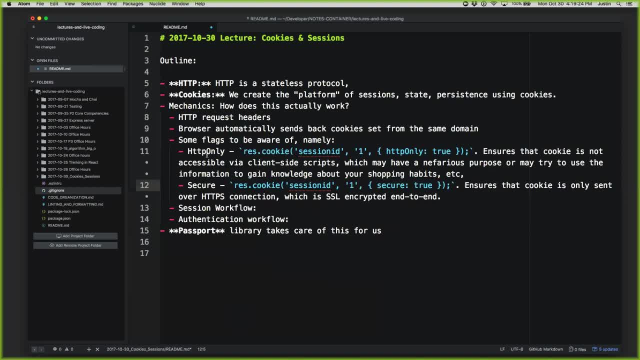 And that says: only allow access to this cookie on the client side, on the browser side, from HTTP. Don't allow access from JavaScript. And one of the things that prevents is malicious JavaScript from accessing those cookies and fiddling around with them when really you might only need the cookies to just be sent. 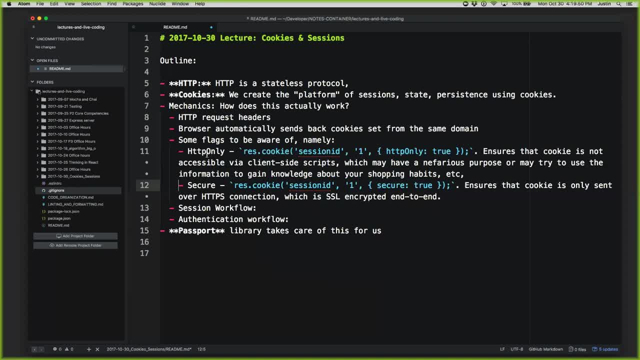 back and forth from the browser. You don't need JavaScript on the client side to be accessing them at all, Right, So this is oftentimes a cookie that you'll set And then secure. This says: only send this cookie if we've got an HTTPS connection. 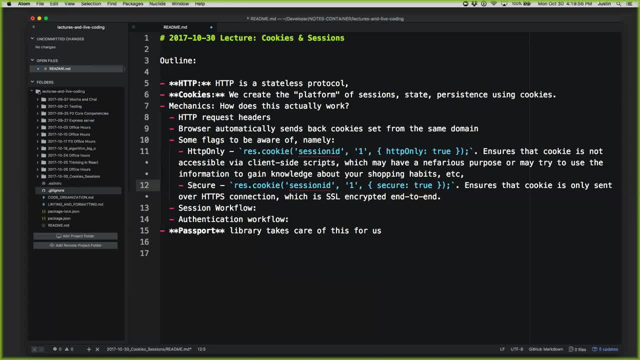 And in my recollection we don't work with HTTPS connections much. I kind of wonder in Express if it's as simple as like plugging in some middleware or like a base connection or something like that. I don't know. 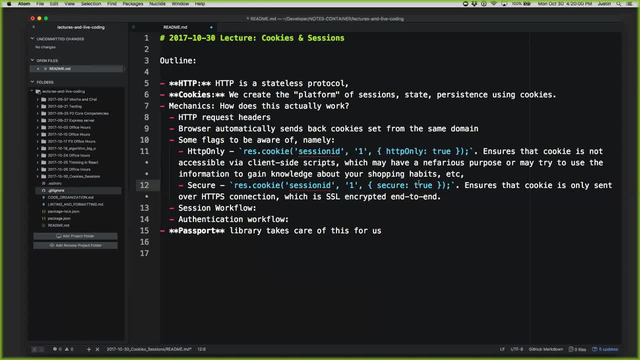 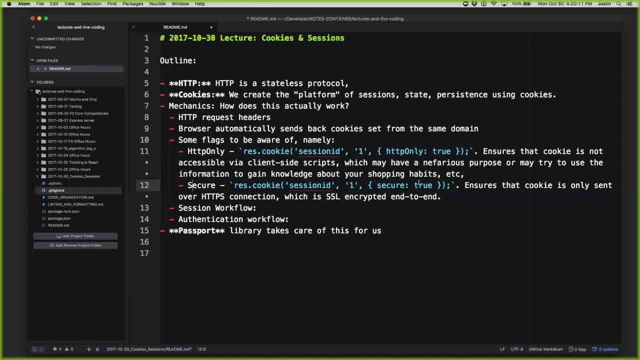 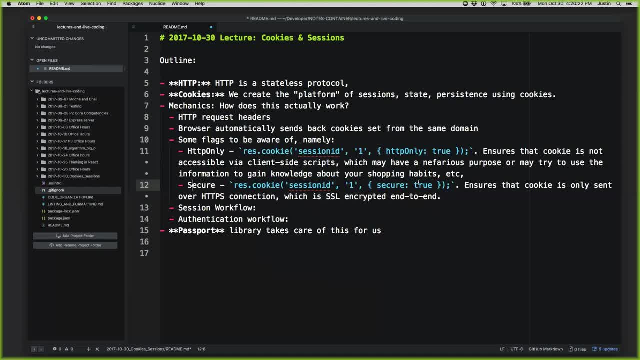 I don't know, But just know that in the wild, out in the wild, you will probably want to be setting the secure flag for your cookies, Because otherwise the cookies will be sent over just HTTP, which is sniffable Like it is. 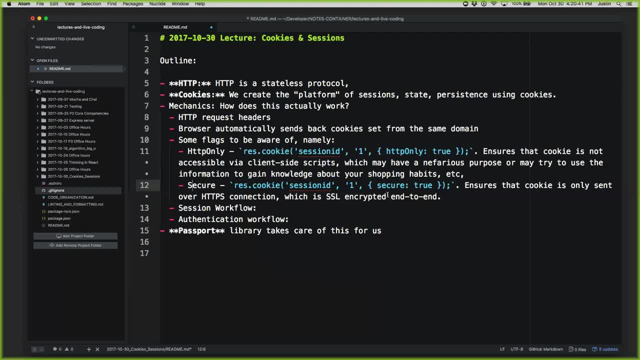 If anybody saw the packets, they would know exactly what's in the cookies. So that's another reason to make sure that you're encrypting the sensitive information that's in there. Yeah, so then? so that's the actual like cookie kind of mechanics. 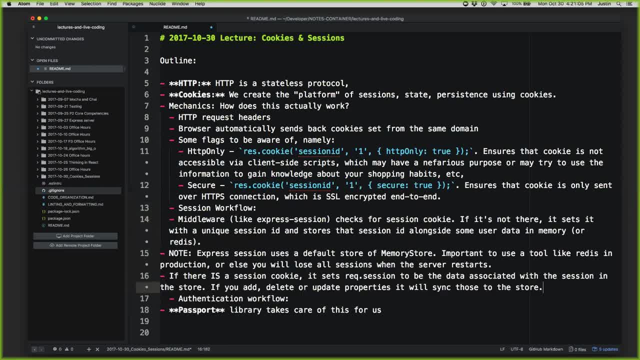 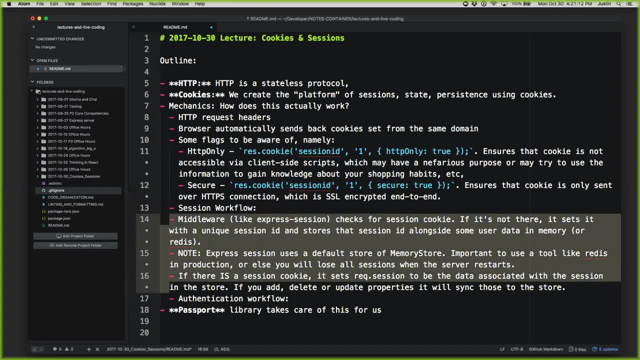 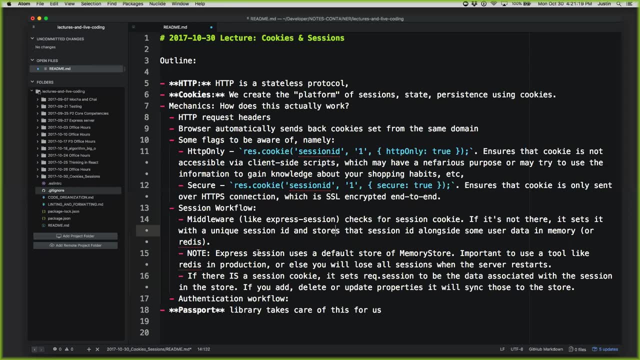 But if we're talking about sessions, So sessions, We usually implement those with Express, with middleware. So a library like Express Session will check for a session cookie. So it checks to see if the cookie that it usually sets is already there And if it is, if it's not there, it'll set a cookie. 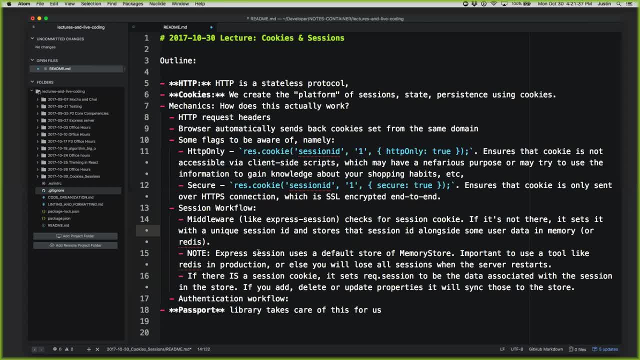 Giving it a unique session option, And then it stores that session ID that's encrypted, And then it stores that session ID alongside any session information in memory. Right, that's what we were talking about earlier. Yeah, and so then, if there is a session cookie- which there either will be before you start or Express Session- will set one right after the first request. 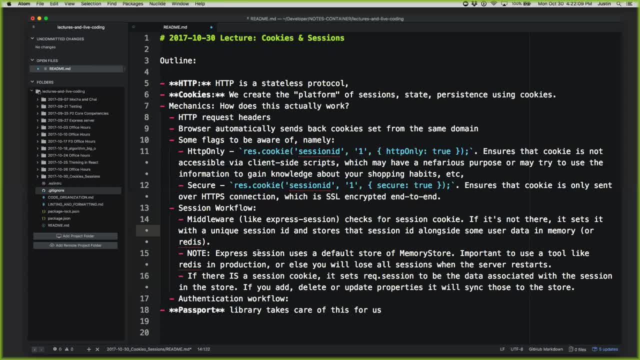 Then Express Session sets RECSession to be the data that's associated with whatever session you've got in the store, So you can add things to RECSession and it will pull those things back up every time a new request is made. So that's what it's doing: to create the experience of a session on top of the stateless protocol. 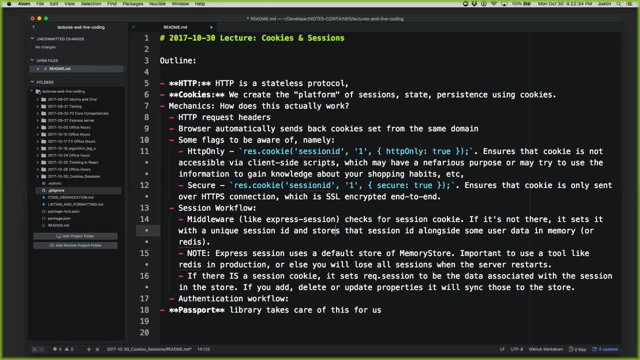 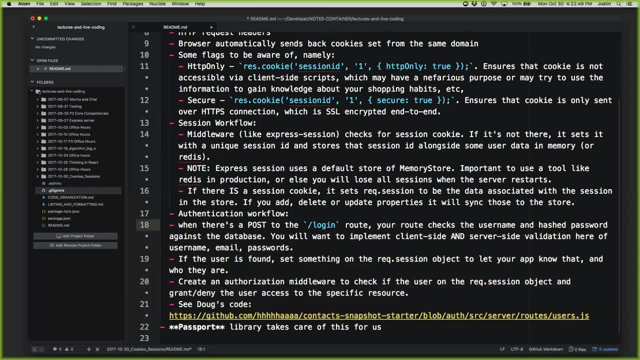 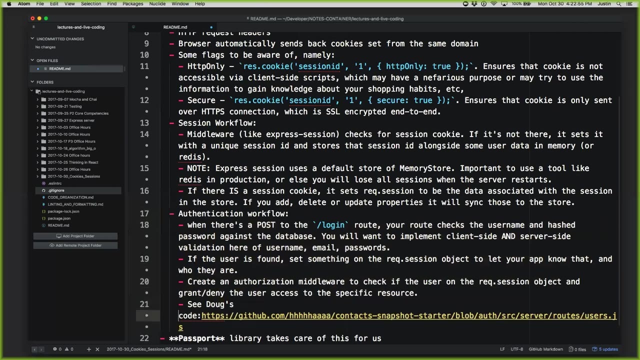 Yeah, and then just to add to that, Yeah, Yeah, And then just a high level, look at like what an authentication workflow actually looks like, And again you may have built something out like this. So stop me if you have questions or disagreements or whatever the case may be. 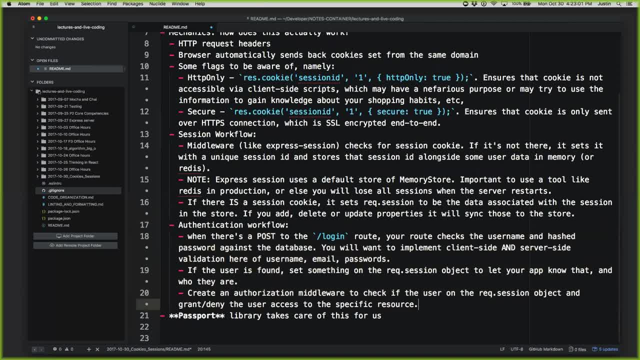 So you have something like a login route. When there's a post to that, your route checks the username and hash password against the database. This is the place where you want to implement both client-side and server-side validation. So server-side, so that you can ensure the integrity of your information. 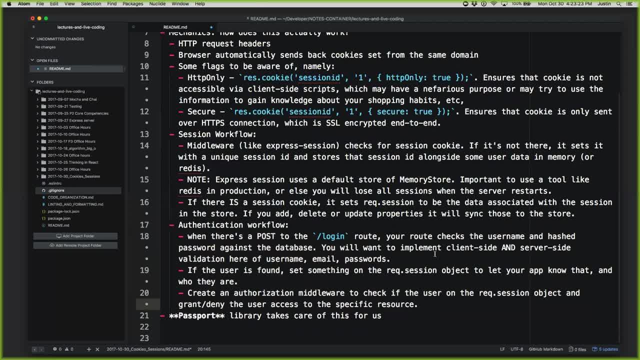 Client-side so that you can ensure people haven't made dumb mistakes or put their username in the email field and the email in the username field. So there are plenty of libraries to do that. Have folks done front-end or back-end validation? You've maybe done something basic like: has anybody had a sign-up form where you collect two versions of the same password? 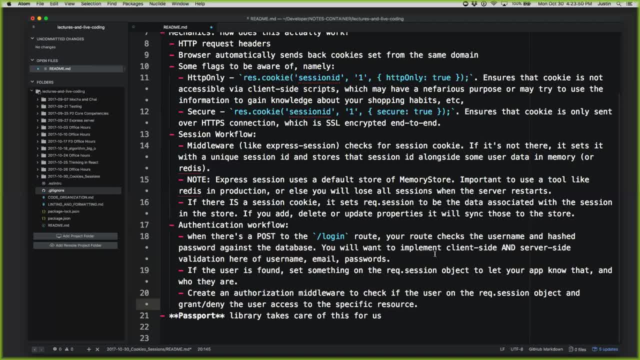 Yeah. And then on the back-end you check them to make sure they're the same- Yeah, So that's one example of it. And then things like checking to make sure the email is a valid email, Checking to make sure your password is valid. 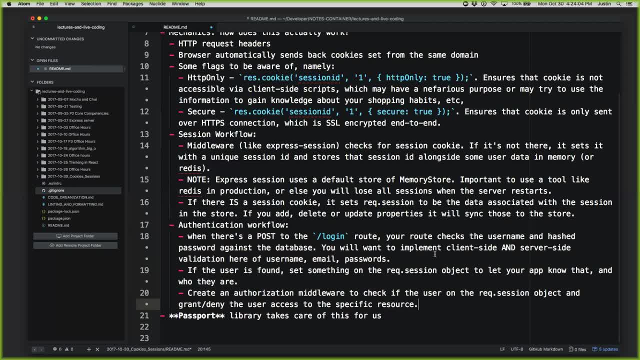 Within the constraints, you say So like letters and numbers, but no special characters and no spaces, And you know like all of that stuff is stuff that you'll want to be checking when you do this Like regex- Yeah, You could use regex. 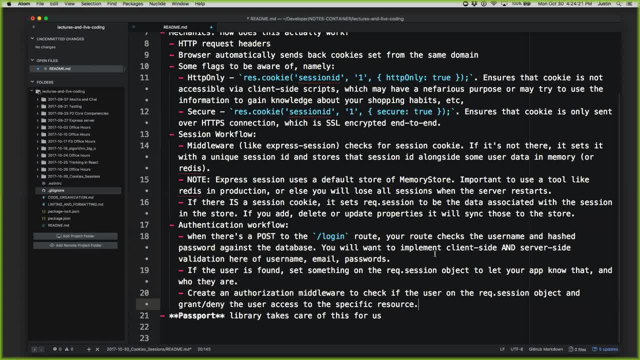 But there are so many good developers making good libraries that kind of like: take care of that for you. I'm trying to remember what one I just heard about was. I'll think of it. But so there are a lot of good libraries that you can just use that, because you would have to build a regex. 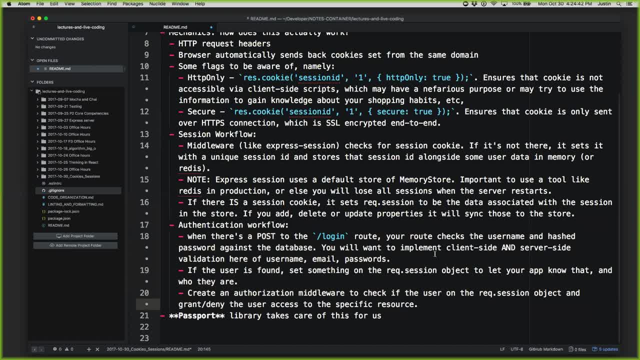 Like everybody knows what a regular expression is: regex. So to create a regex that successfully identifies all email addresses and doesn't misidentify any, it's this like. I mean. it's like just a long-ass thing Because there are so many different kind of caveats and special cases and regular expressions are not the most like terse way of you know, checking a piece of information. 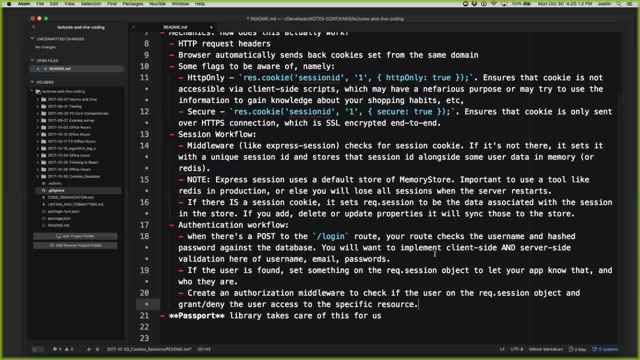 So I'd much rather rely on somebody who had come up with some- whether it's a regular expression or they have some other way of testing the email address, for example, And that they've tested it and a thousand other developers have tested it and used it. 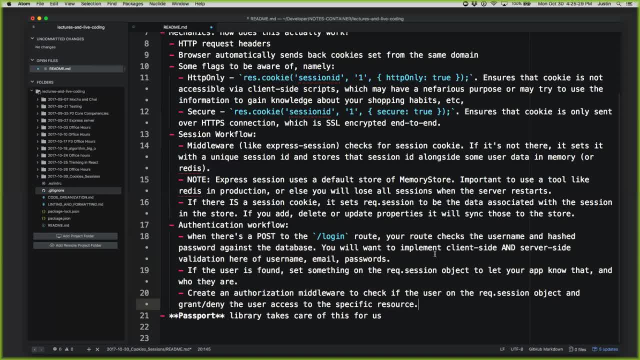 And so now it's a library. So yeah, And that's true on the front end and the back end There are front ends. There may be front end specific libraries for this kind of validation, But you know, in general you can use the same sort of thing. 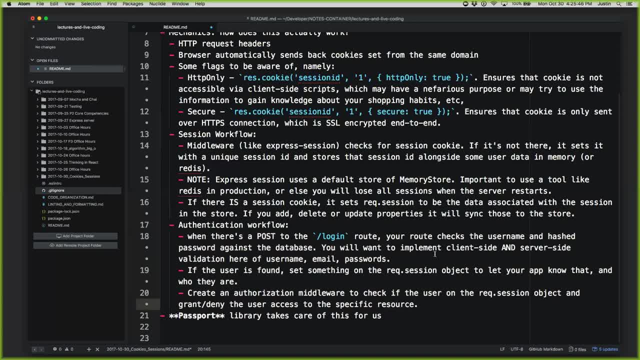 And the front end validation is nice, just to give the like to give the user a nice and kind of fluid experience of what's going on. So if you didn't type in your password correctly the second time, it's nice to know that right away. 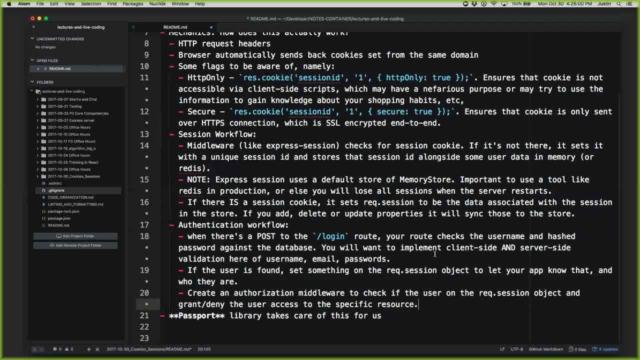 Rather than later. But then after you hit send and you get a response back and it says there's something wrong with your form, and then half the form fields have been erased and they have to, you know. You know what I mean, Yeah. 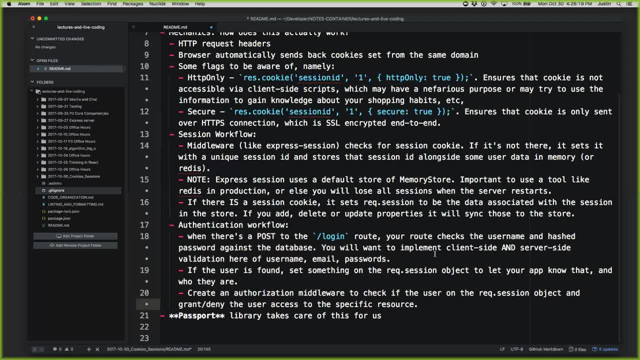 So Yeah. So if the user is found, you might set something on the recsession object To let your app know that That could be a user ID. You could put any amount of information that you want on there, And then you'll have some sort of authorization middleware to before you serve up a route. 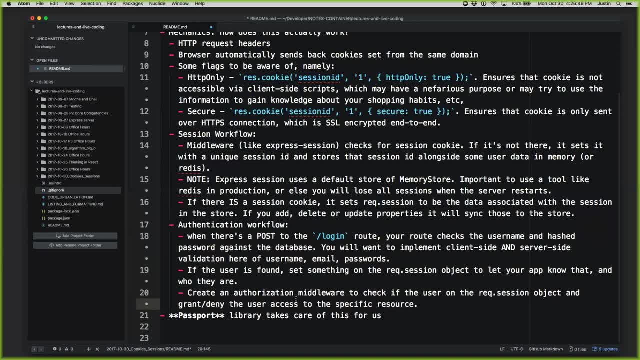 So like, if you have a route that's like slash protected secret information, you would have some sort of middleware that runs before that that says is recsessionuser or user ID or something like that set. If so, and if they have permissions for this thing, then great. 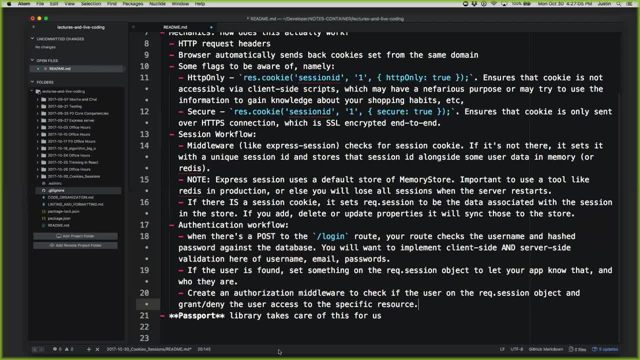 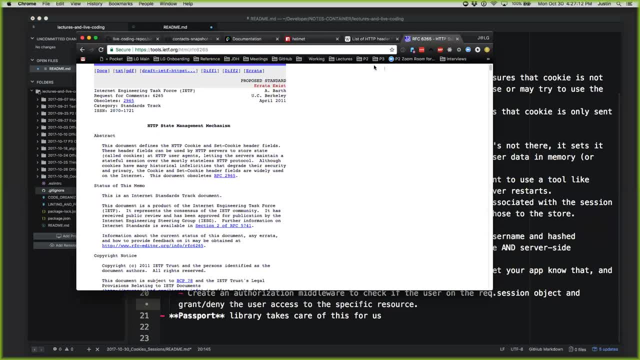 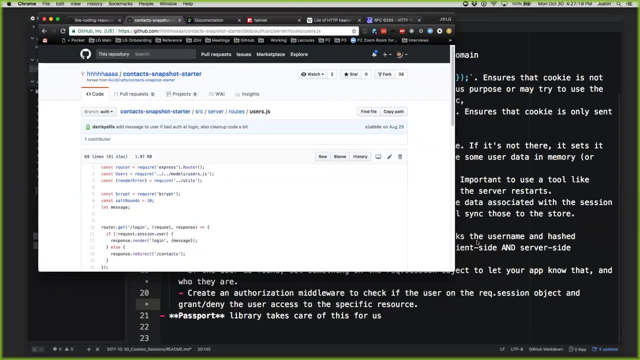 If not, then not. And just to get us looking at a little bit of code Doug Leboway had a great, great version of I think this is the contact snapshot like authorization goal, And I just wanted to point to a couple things in this. 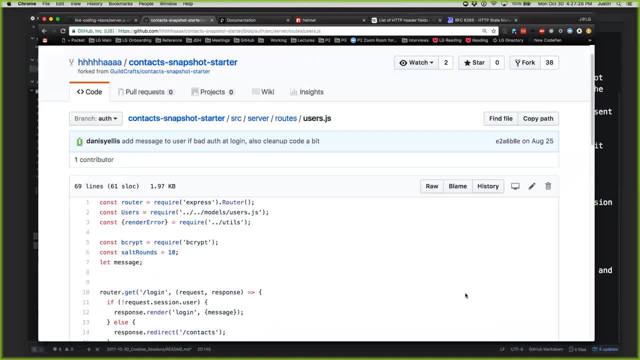 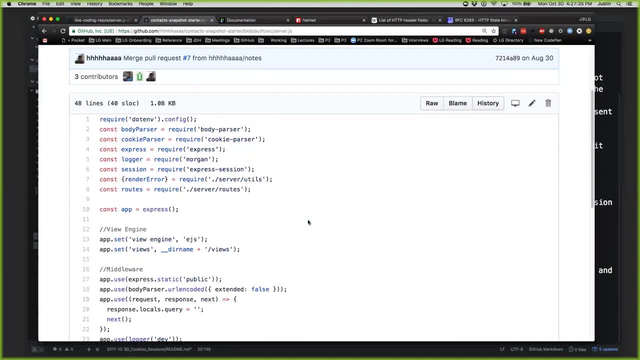 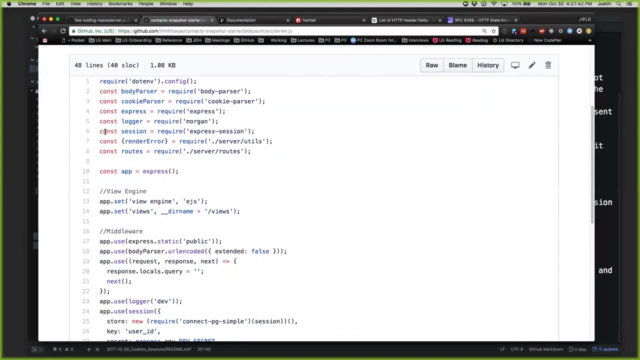 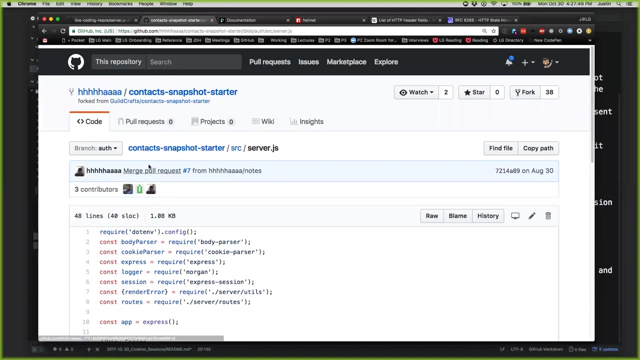 Let me make this a little bigger. So this is the users, But I'm going to source server. So normal express server. We're using express session here on line 6.. But most of the most of the actual magic happens in is: 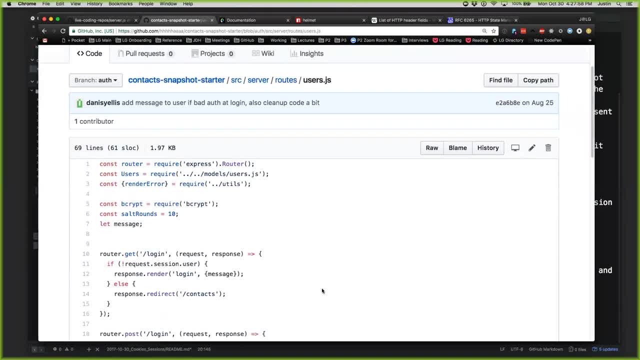 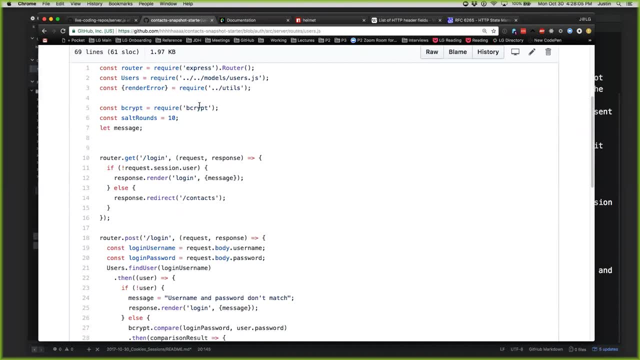 Routes And I think it's users here. So the only comment I would make about this code: that's really good. I would make sure to put bcrypt in my like models side of things. So the MVC Bcrypt to me belongs like somewhere in the in your model so that you can just call a function of your model that's like you know, check and see if this person is in the database. 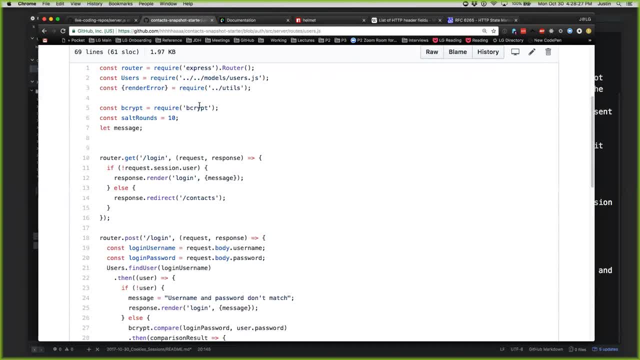 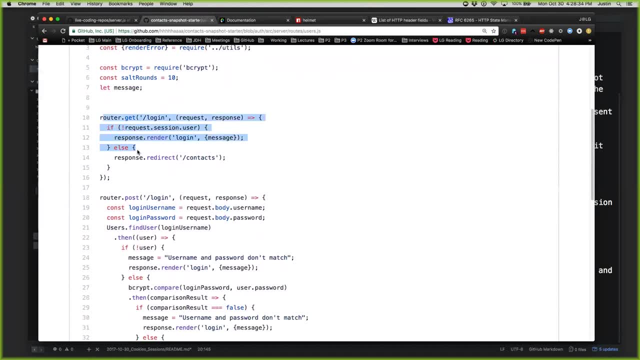 And then that's actually running the bcrypt, compare or bcrypt hash functions needed to do that. But right, so you've got a login route And if user is not set, then you can go ahead and render a login. If it is set, then you redirect here. 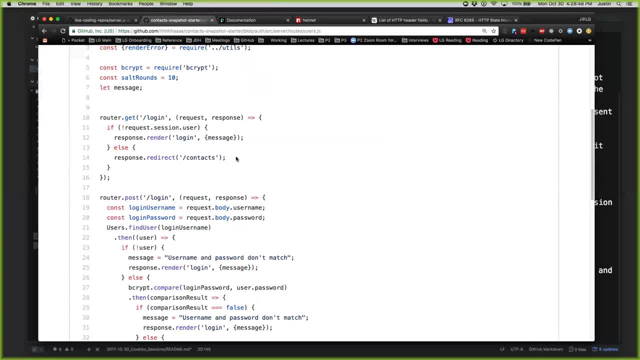 I wouldn't necessarily do this particular thing, Like if I have a web app and someone goes to the login page and they're already logged in. I don't know, I could see reasons to do both, But I might actually show them the login page so that they can just log in again. 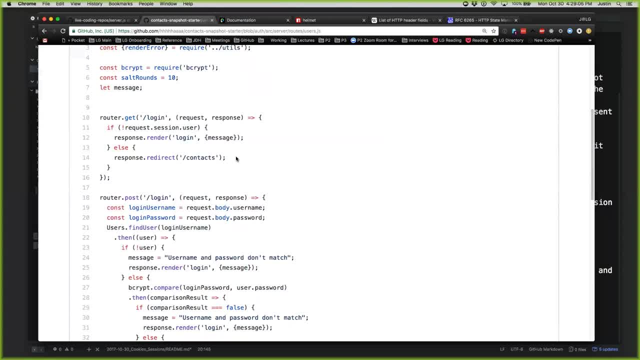 Or I might show them a special like log out button that says like hey, you're already logged in. You know, do you want to log out Right? Rather than every time you click the login button, it redirects you to a different place. 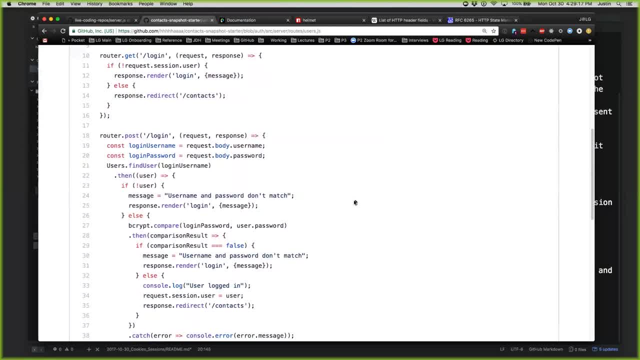 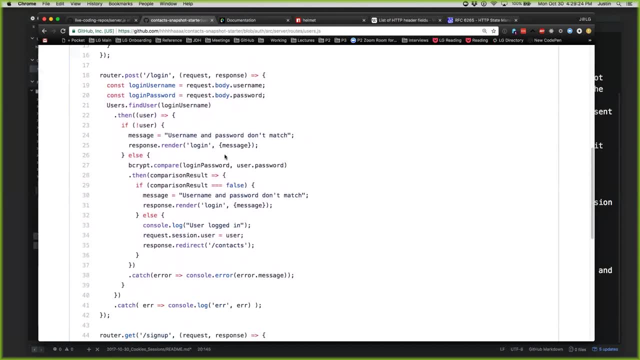 So just a small thing. But then when you post that login route You get the username and password off the http form body. Can you see this okay? Yeah, I can tell that it's the afternoon, Like in the morning. this group is like bright eyes and sort of like totally. 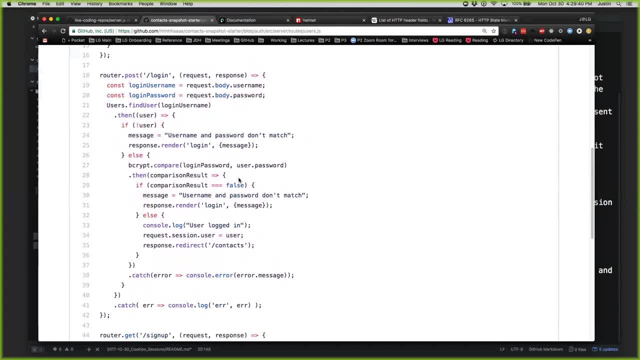 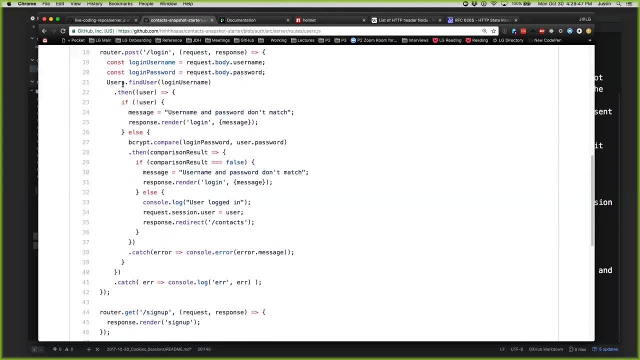 And everybody's kind of like It's pretty cute, Yeah. so then you go to the user, To the database. You try to find that user. If you don't find them, then you have them log in again. What's that? 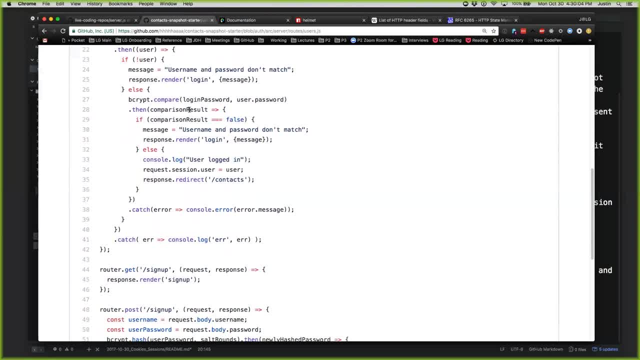 It's all right. It's all right, And otherwise you do this. bcrypt compare. That's the function that will look at your hashed password and the unhashed password And it knows how to compare those. Incidentally, do you know how that works? 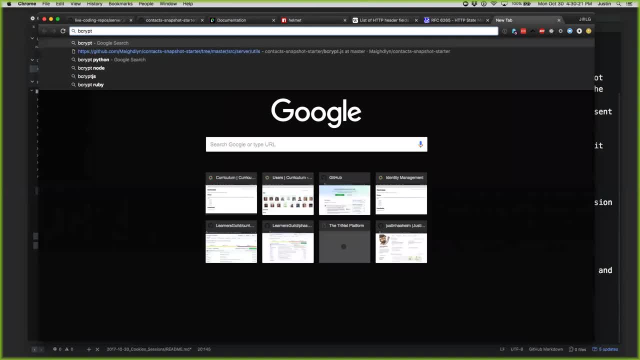 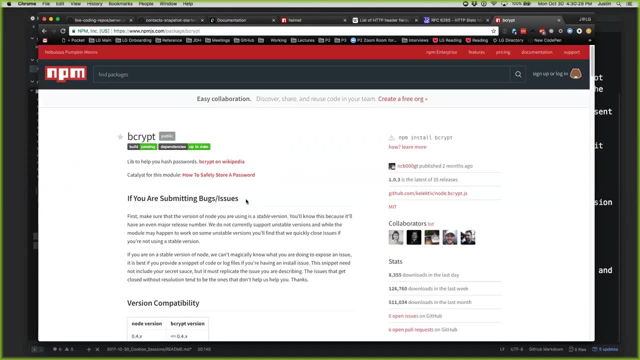 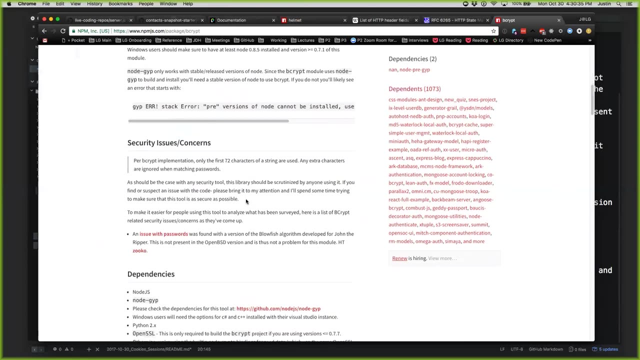 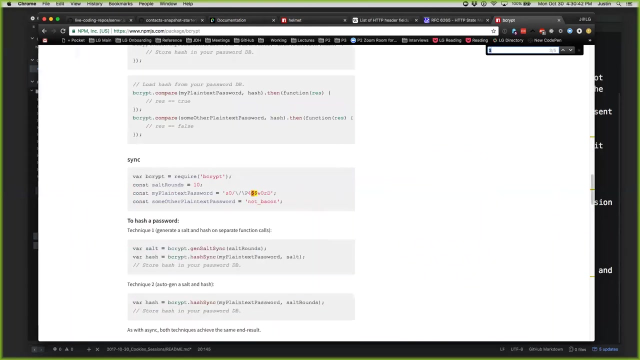 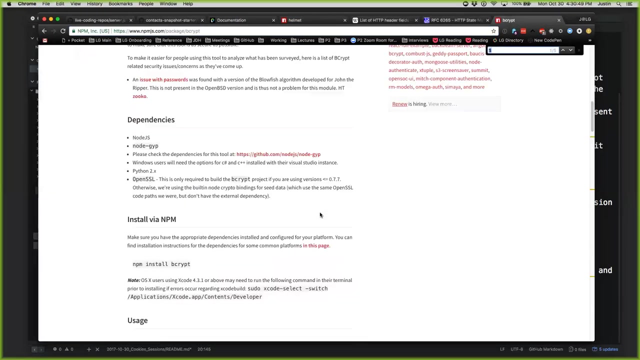 That, like a bcrypt Bcrypt, A bcrypt hash password actually includes the salt and the number of rounds in the actual string. Have you seen this? Let's see if I can find it. Yeah, Yeah, it's not going to show it to me. 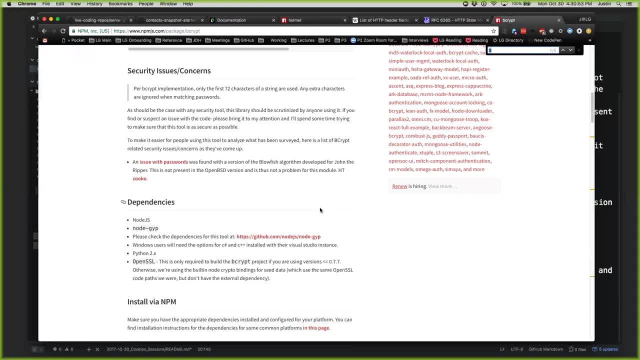 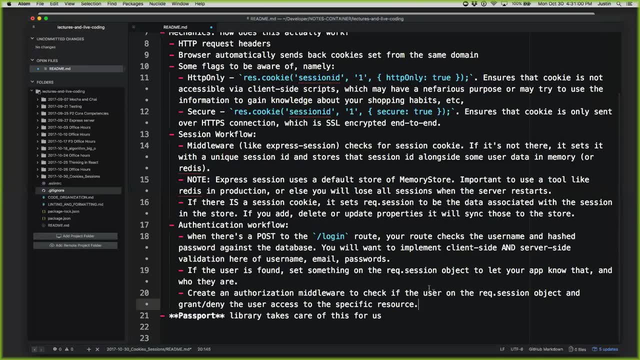 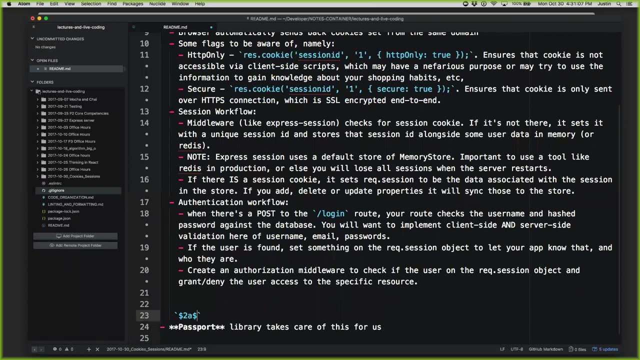 But. But if you do this, Like when you go back to whatever you're doing, look at hashed password that you see in the database and it'll be something like: It'll be something like $2A, $10.. 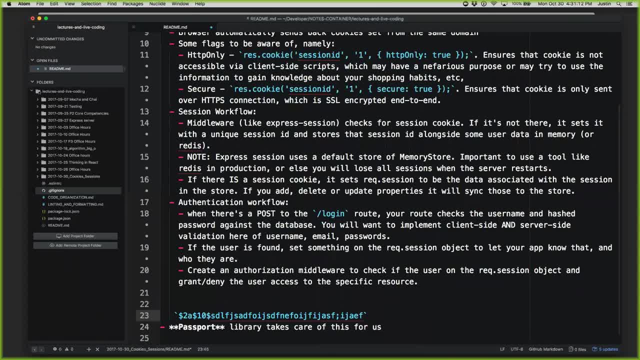 $A bunch of extra characters And the dollar signs are delimiters. that I think. the first thing is the salt, the second thing is the number of rounds, and then the rest is the actual number of rounds and then the rest is the actual hash. yeah, there we go. so that's. 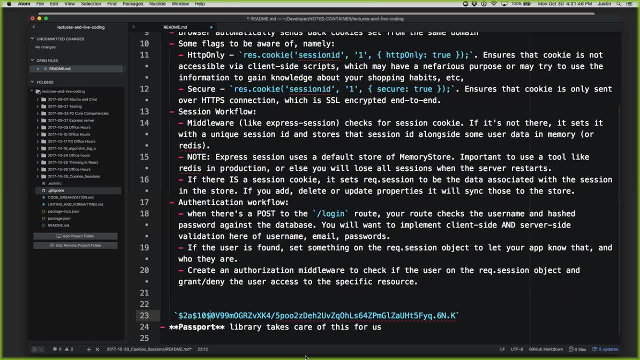 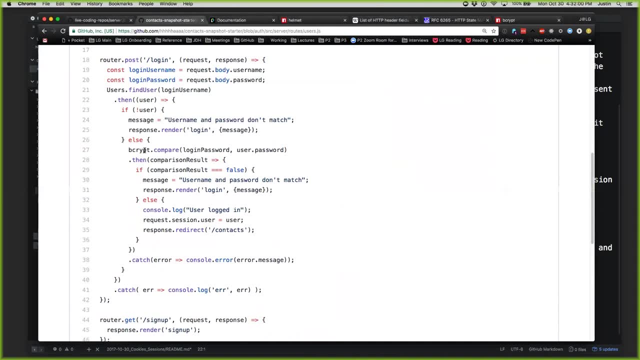 how big rip knows it. it basically just decodes that and then it's like: oh okay, 10 rounds. oh okay, here's the salt, great, yeah, so back to the code. for a sec, say again, I would pull this be grip logic out of the route itself. but if the 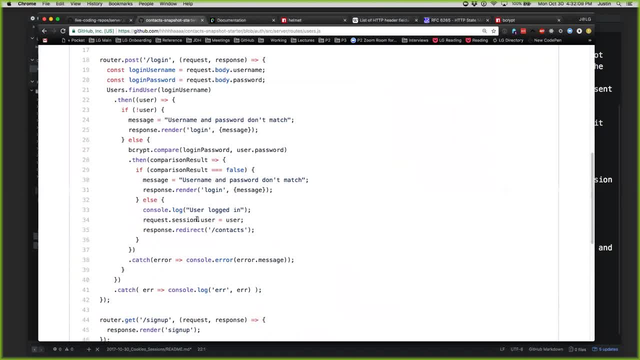 comparison is true. then you log the user in and you do that by setting wrecked out session that user to the user name, right, and that's just like you're internally identified the user name. and then you log the user in and you do that by setting. 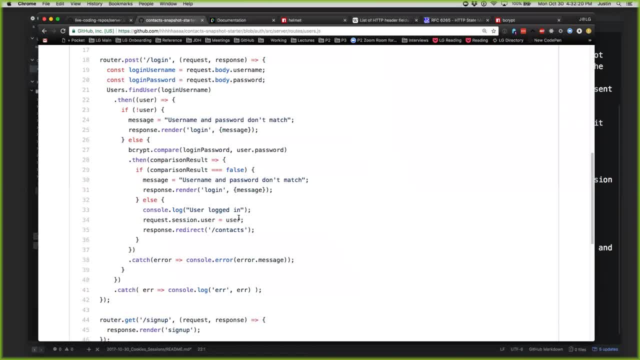 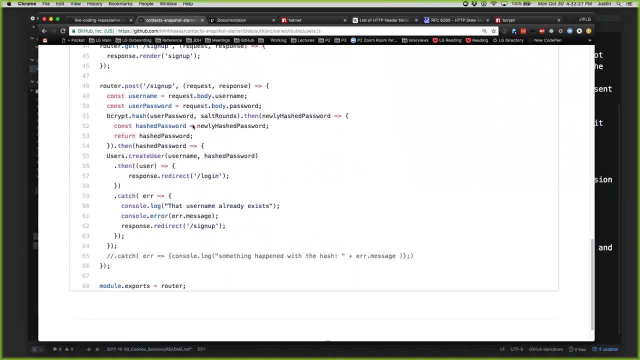 that thing where you're saying: when that's true, we know that somebody's logical, yeah, and then the sign-up route be familiar. if you've done this, benchmark is you get the username and password off the body again. you might get a password and like a password match, off the body so that you can compare the. 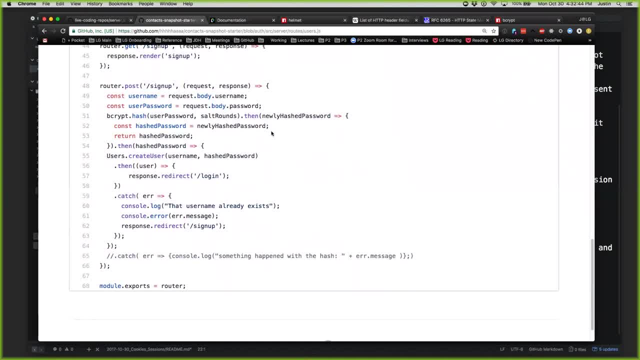 two and make sure they're the same. so then we're at the end of the session and then we're going to go ahead, and so then we're actually hashing the password with however many salt rounds we have and taking that hash password and somewhere in here. yeah, then putting. 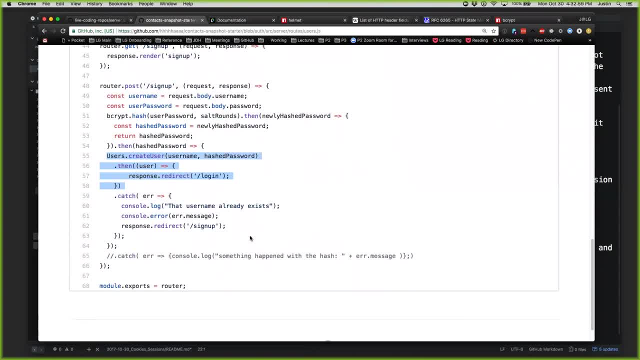 it in the database and then you can redirect someone to sign up or you can just call them log in. I don't know if there's some like best practice about that. I feel like some. some websites you'll sign up and then I'll say, okay, now sign in. and some websites you'll sign in and 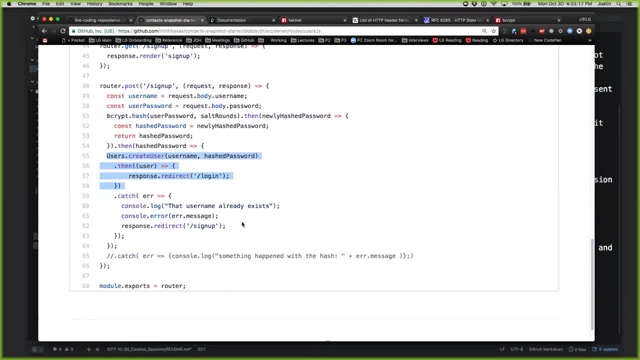 And some websites. you sign up and you're just in right, Yeah, Yeah, That's interesting. I don't know if there's like some compelling reason to Sure, Sure. So if you have some multi-factor signup workflow where you're asking people, 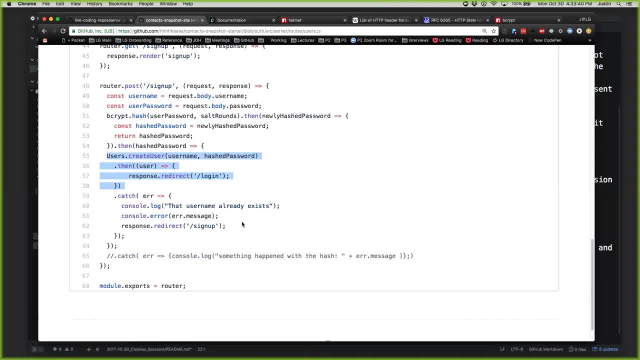 to confirm that it's a real email address, which is good um um, from like a business marketing perspective, because you want to make sure that people are using real email addresses that you can spam mercilessly. but it's also good from a- I mean good. 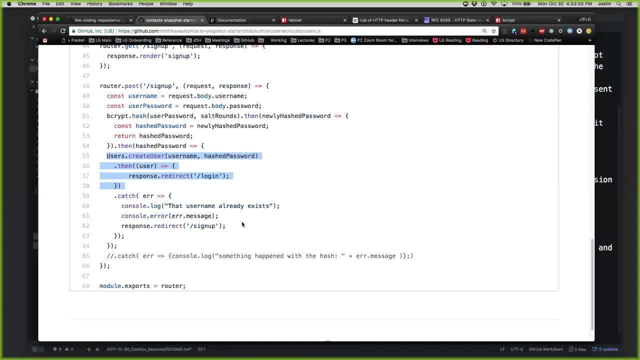 It's um, it's also good from the perspective of you want to make sure that they entered the email address correctly, And if they don't get the thing, then they'll know that they didn't enter their email address right. 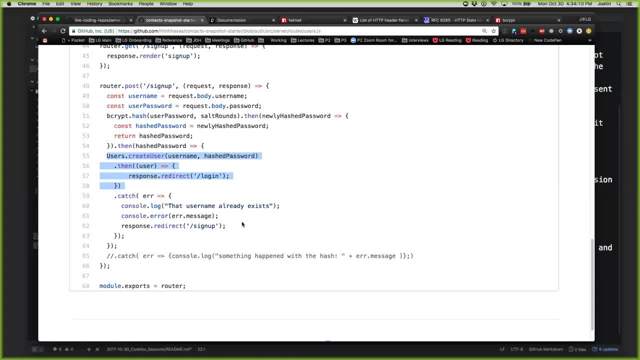 You know the way to get around that if you're signing up for a service that you you really don't want to be on their email list. Uh, I don't know about bug me or not. What's that? Um, it's a website that for for most websites, 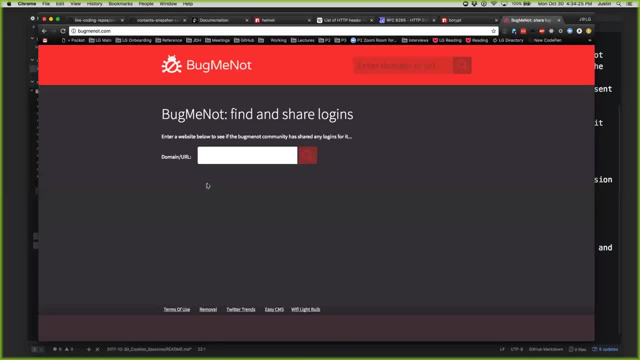 users will post, just throw away emails and passwords. Oh yeah, Oh no. So like um Netflix and services that you have to pay for, I'm usually not one to help. Hi Yeah, I wonder, like um chesscom. 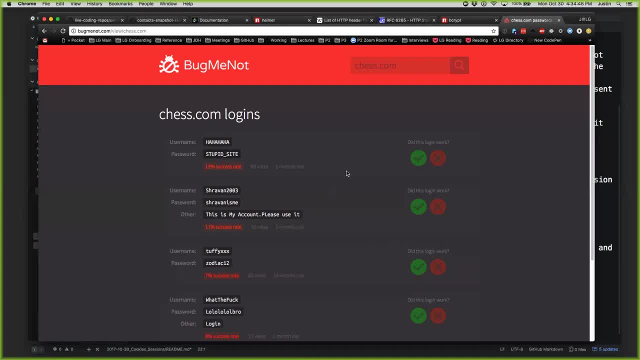 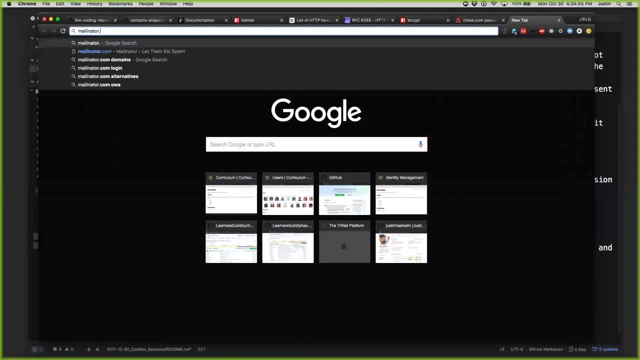 Yeah, Yeah, There we go. Password, Stupid site, Yeah, So the one, the one that I use- is um mail in nature, and what this allows you to do is you can create any email address that you want. That's like you know. 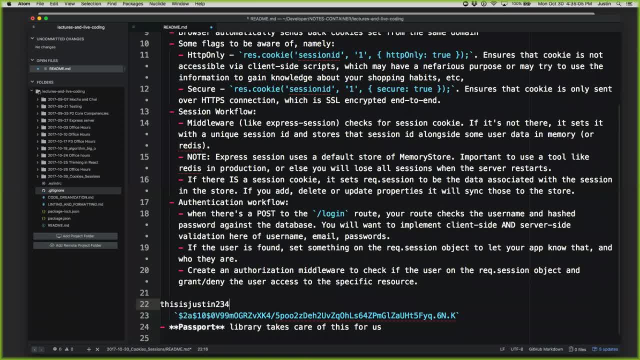 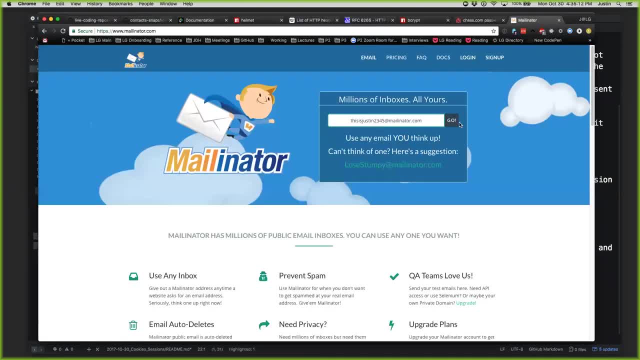 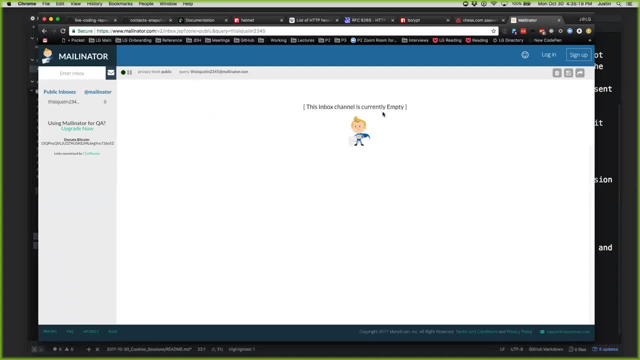 this is Justin: two, three, four, five at mail in naturecom. And then you can just go to to mail in nature and say: I want to check that email inbox and it'll say: great, here you go. Uh, no emails. 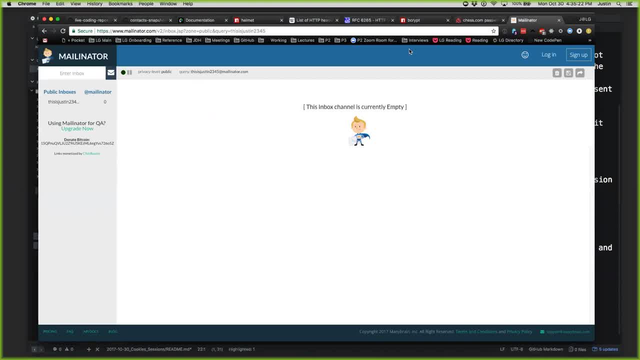 But if somebody sent an email to that address right now, it would show up in here. So their idea is: like: all of their email addresses are publicly accessible, like and, and you just you want to use it in the isolated case where you're like signing up for. 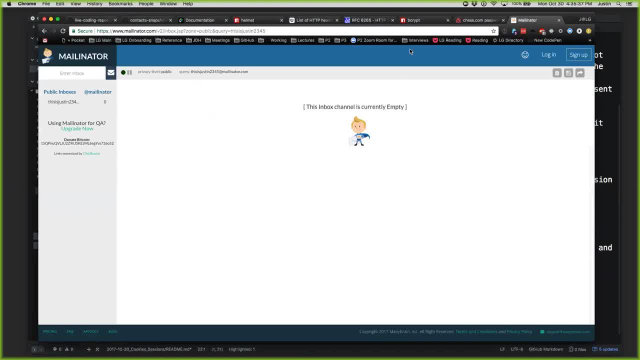 something and then the email gets deleted after like a couple of days, Um, but it's kind of a fun solution to it, And so they have um mail in naturecom. but because that gets blacklisted from services a lot, they also have other. 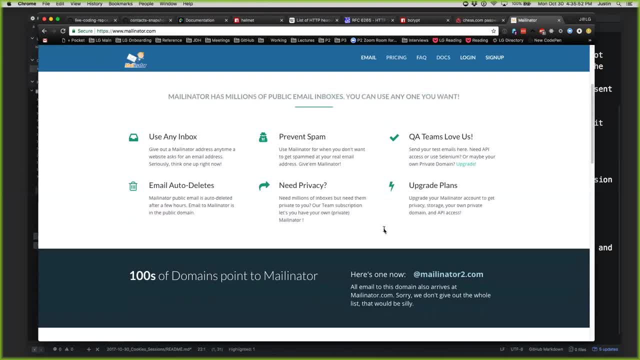 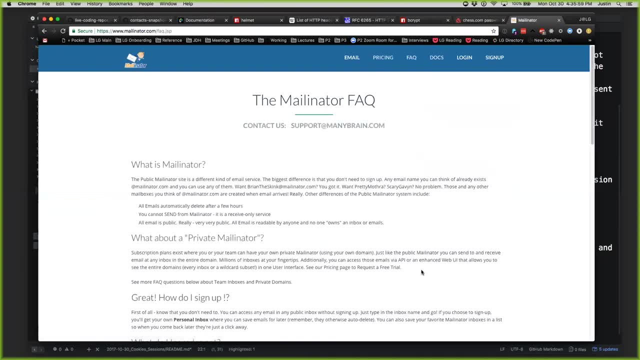 um domains that you can, where you can do the same thing, And I wonder where they list the domains Um one, but the one that I use, just because it's the one that I can remember, is um Bob mailinfo. 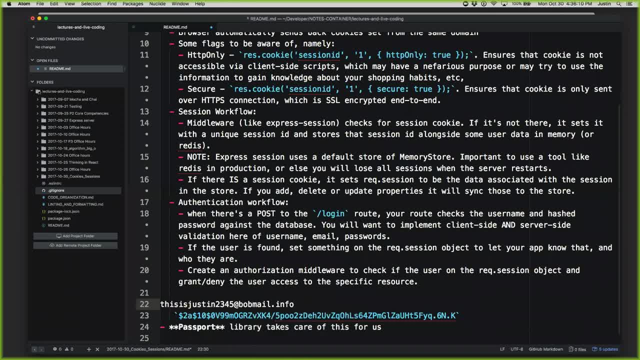 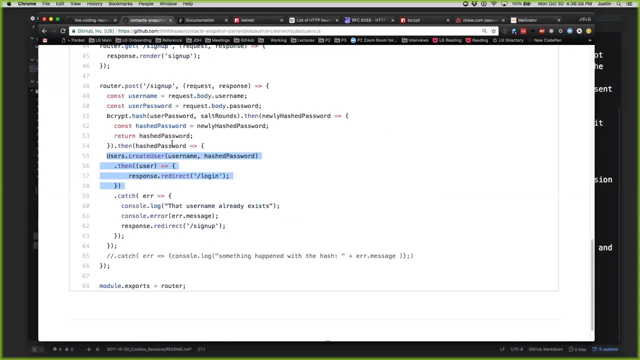 Bob mailinfo And that that email address will go to the same mail inator box. It's like life tips from Justin. Oh yeah, Hmm, Okay Yeah, Um, cool, So, um, come back to the code. 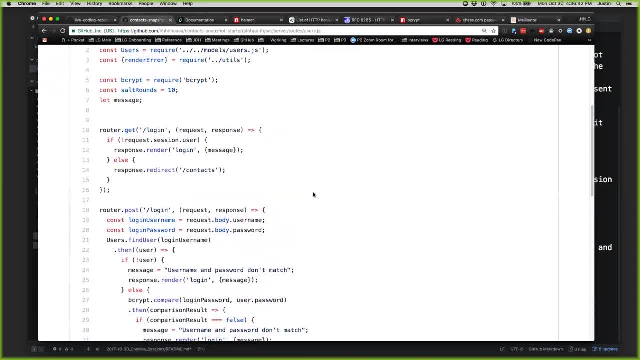 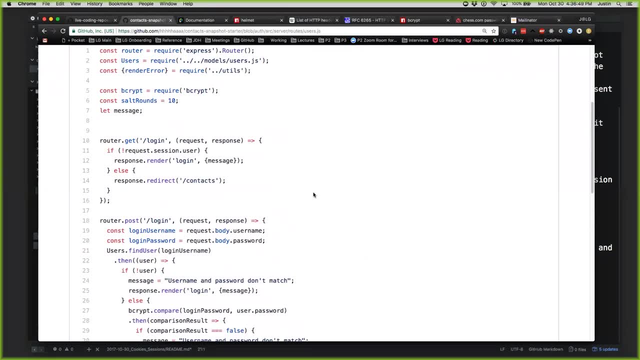 Is there anything else? we want to see Any questions about this code. So this is implementing authorization without um, without the passport library, passport taking care of some of this stuff for us. Show me the part that passport does for you, Um. 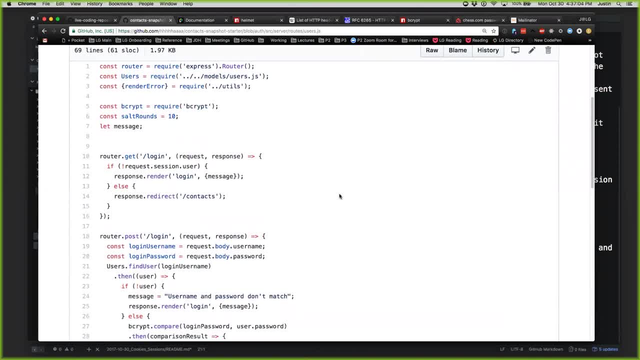 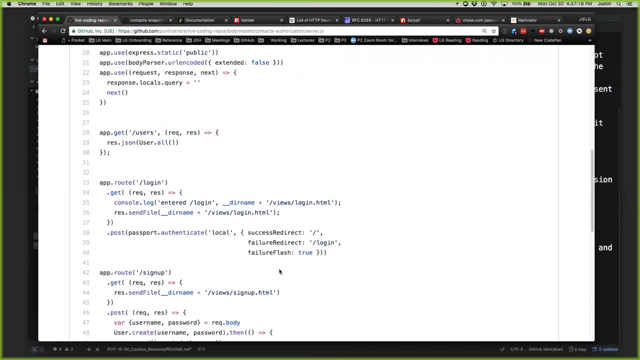 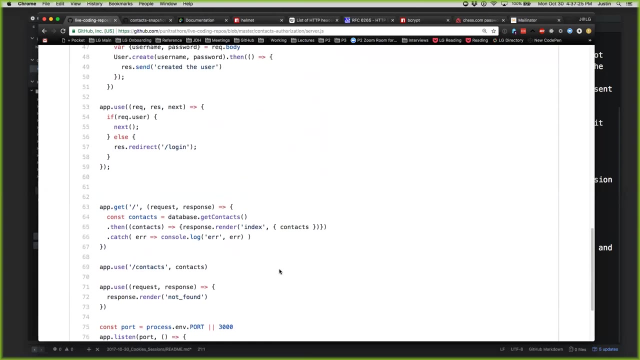 it's like adding the user to the session. Yeah, So what does? what does passport do for you? So, um, this is a different repo. I think Puneet did this to implement passport. So yeah, let's see. 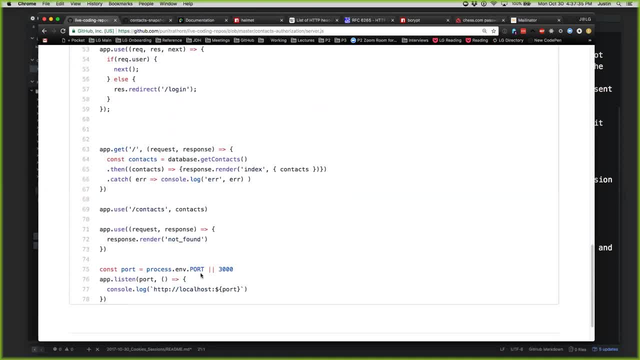 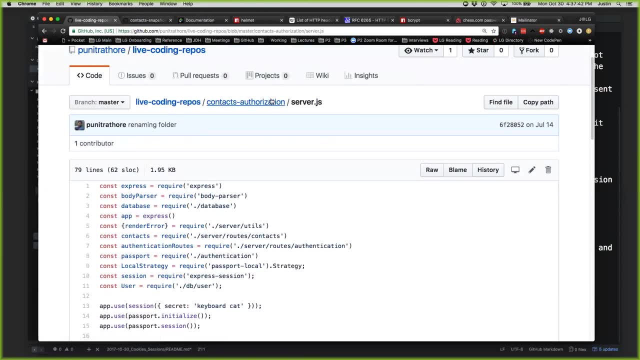 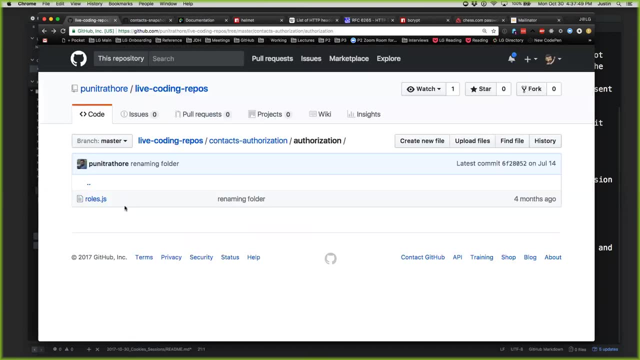 I think the actual passport configuration is in a different file. Let's see if I can find it. Yeah, not this, What's that? I think? uh, on the page you wrote before did it show the um, um? 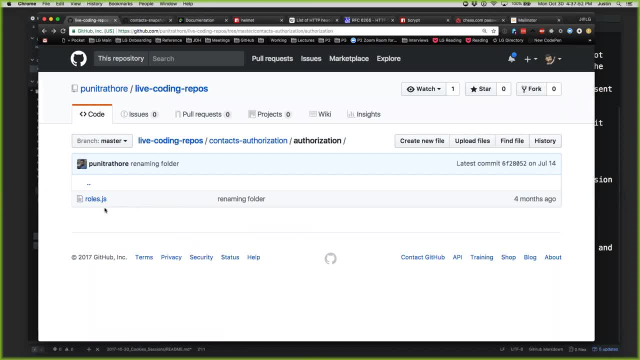 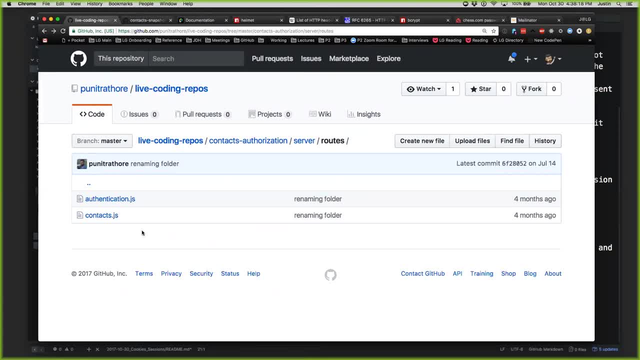 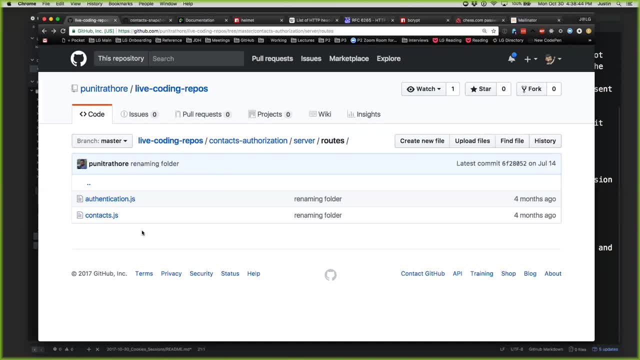 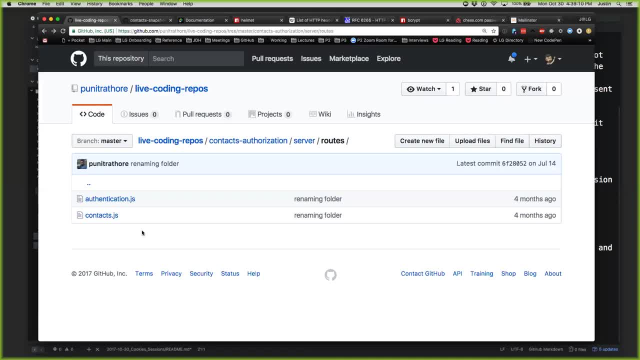 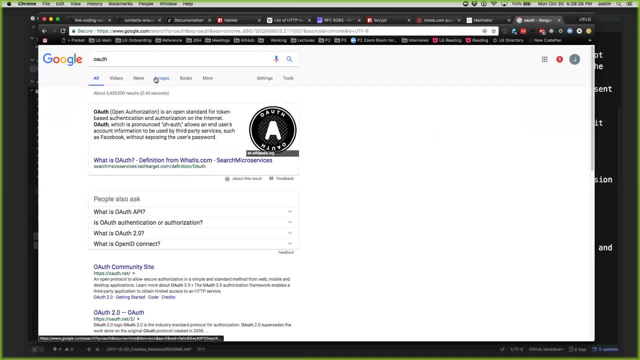 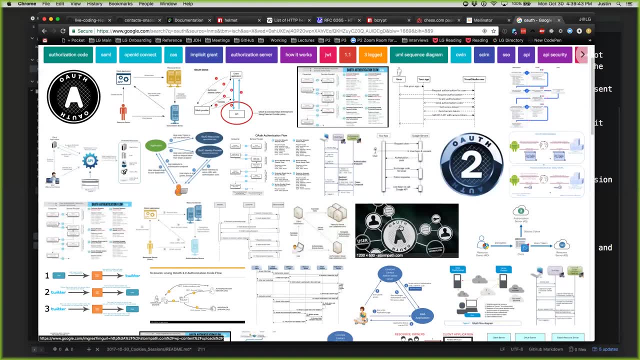 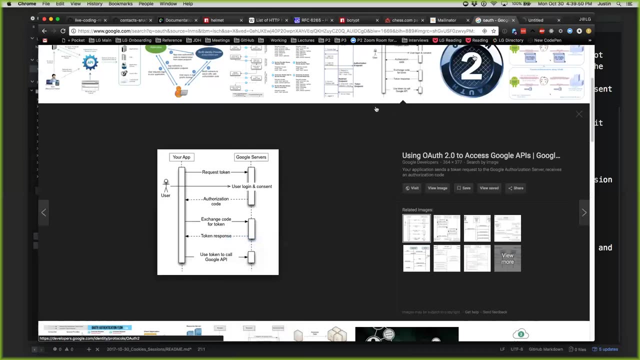 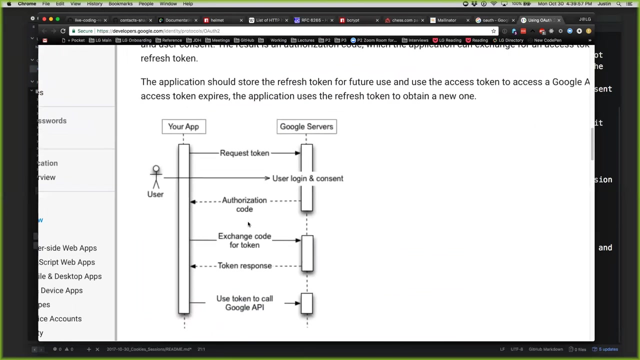 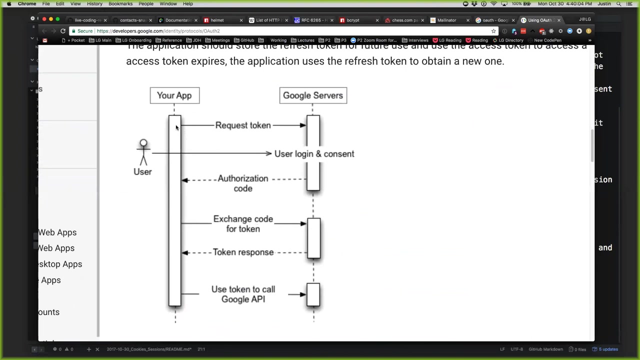 um, um, um gram of what this looks like, since I don't have a whiteboard yet. Not that I'm bitter. This looks promising. Oh, Can you see that? So what happens at first is when you want to log in- so we're going to use Google in this example- you send the person to like. 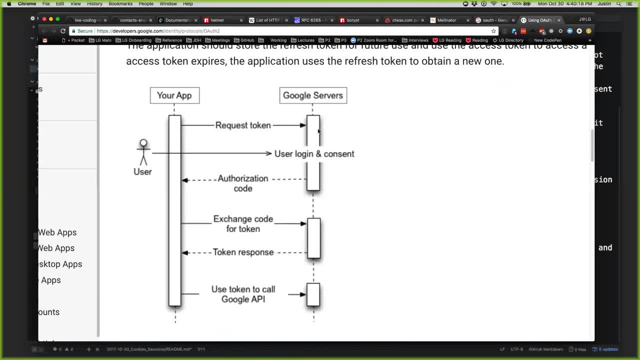 you redirect to the Google OAuth servers and there's a bit of information that you specify with that, including a callback address, And then the Google servers put it to the user. They say, hey, this website X and Y and Z is wanting to get your like Google. 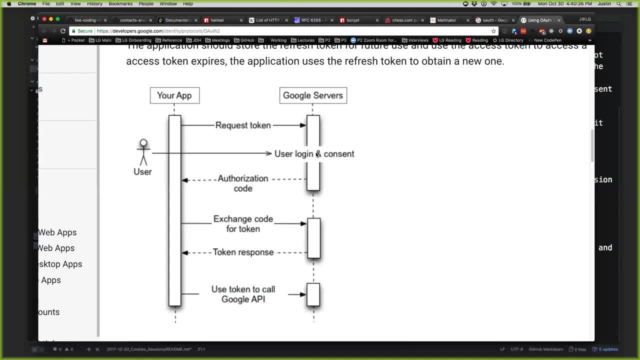 login. Do you approve that? And if so, like what do you do? Like log in here, So then the user will hopefully log in and put their- you know kind of click okay to all of that, And then Google goes to that callback address and sends some sort 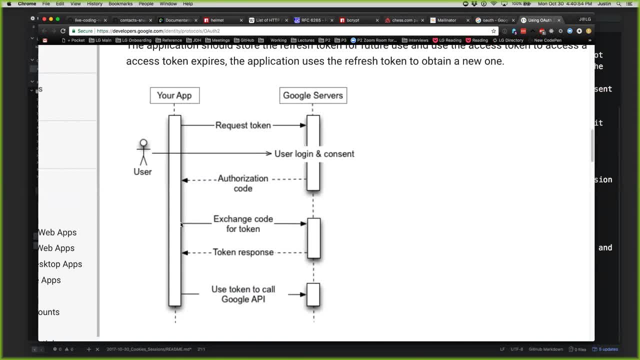 of authorization code And then that authorization code can be exchanged for a token, and I think the purpose of the token is so that you can access like whatever limited amount of stuff that Google has Like. so you might be asking for the person's, just like Google email. 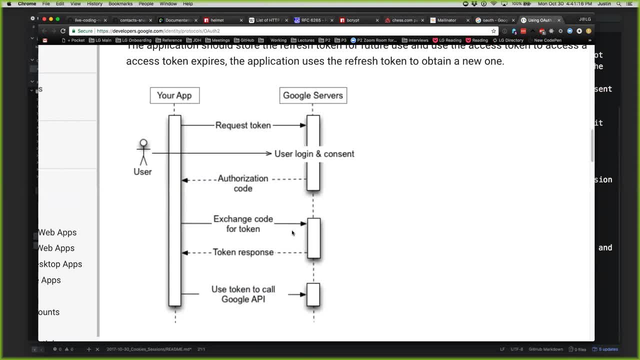 address and like that might be it. Or you might ask for their email address and their birthday and their- you know- Google Drive account access and, like you could, it could be whatever, And I'm assuming that in this diagram that token is used to access those. 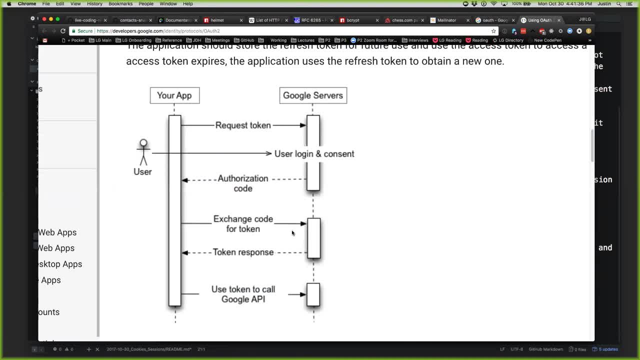 things Okay, Yeah, So, like on your server side, you have a user database that maybe you allow usernames and passwords too, So you allow local login, which is pretty typical also to allow both of them, And so you would have a database that would have a handful of fields You'd 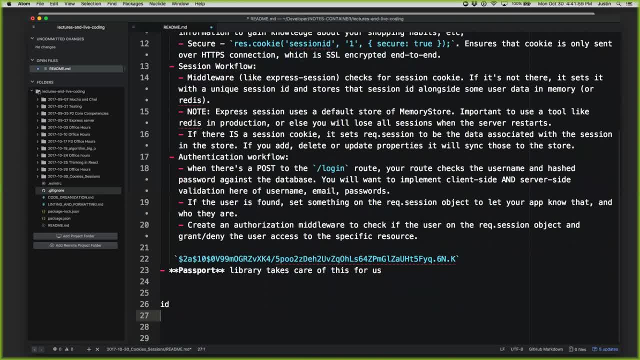 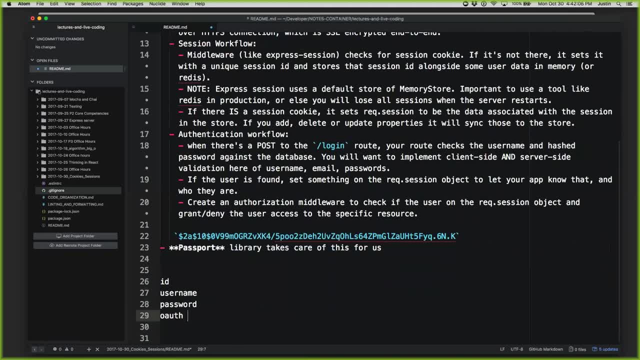 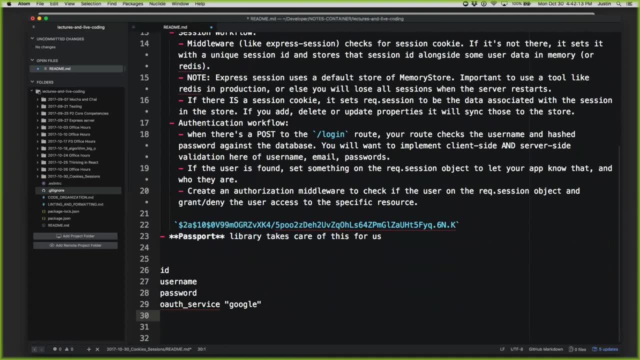 have an ID. obviously You'd have username, password, But then you'll have something like OAuth, Yeah, And then you have like OAuth service And that might be something like Google, And then you have OAuth- what would this be? OAuth like token, What's that? 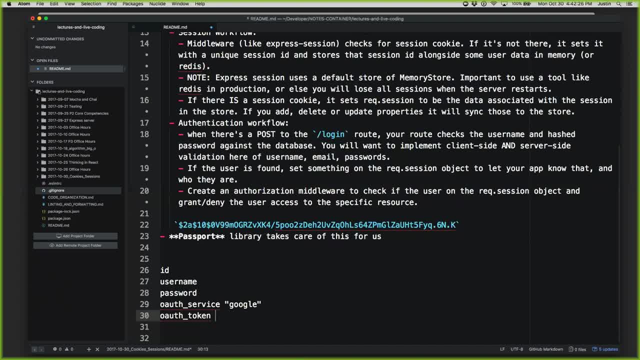 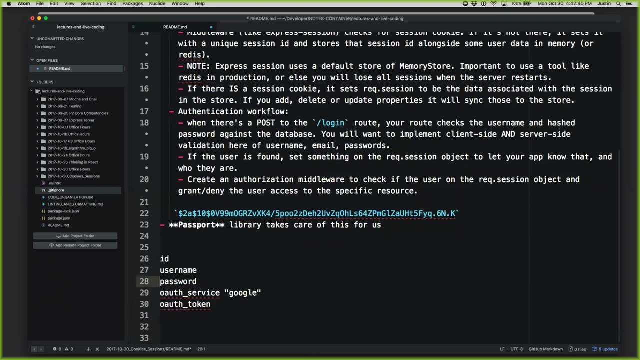 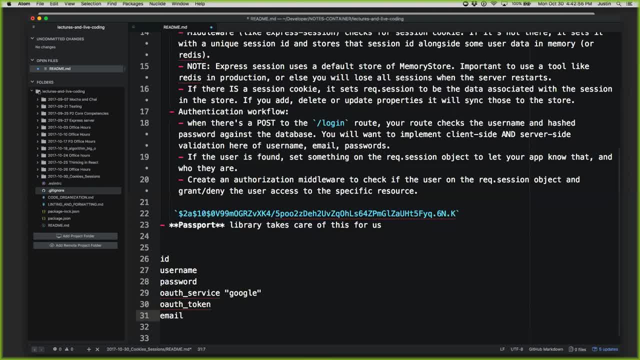 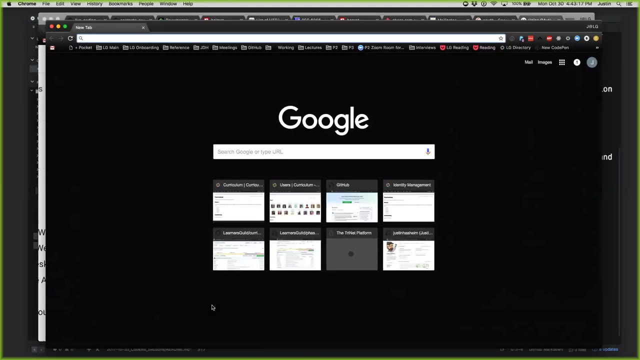 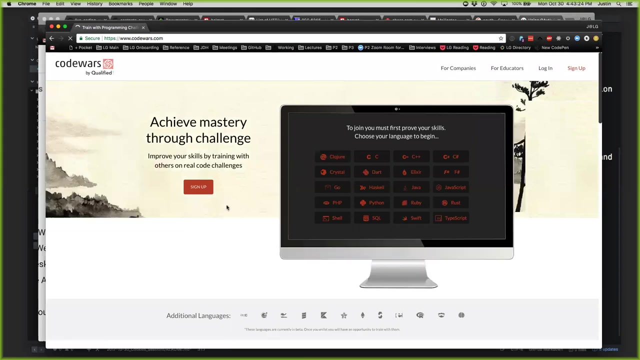 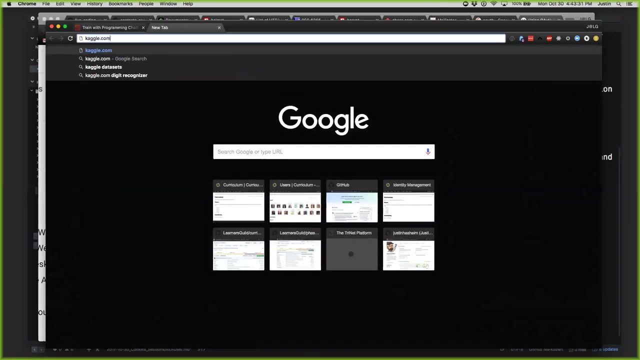 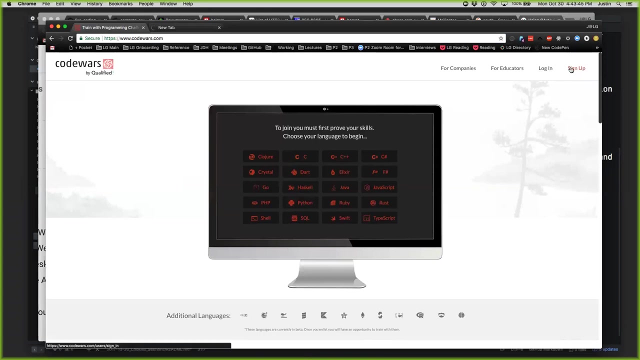 get their email address from you know, from this OAuth service, because that's the de facto way to identify somebody. yes, that is exactly what it is right. so if you go to, that's a good site. that would be an example of this. okay, so you go to login and it says: oh yeah. 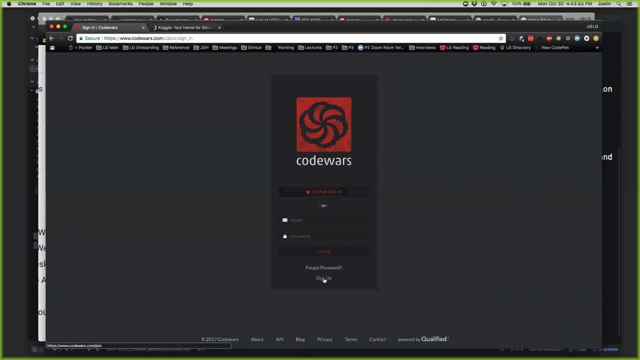 okay, so you go to log in. and it says: oh yeah, okay, so you go to log in. and it says: oh yeah, okay, so you go to log in. and it says: oh yeah, yeah, so that's so, you don't have to. yeah, so that's so, you don't have to. 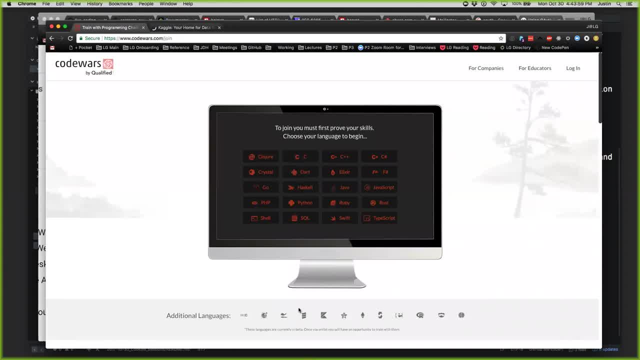 yeah, so that's so you don't have to go through the signup form first to yes. go through the signup form first to yes. go through the signup form first to yes. okay, another site that, oh yeah, like I'm. okay. another site that- oh yeah, like I'm. 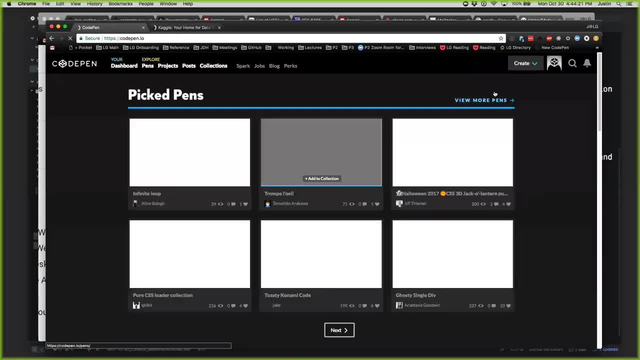 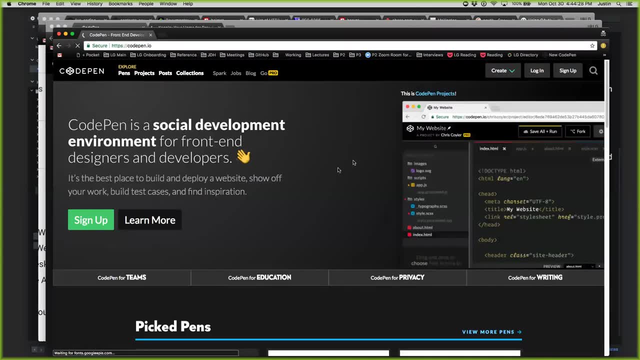 okay, another site that. oh yeah, like I'm coach and I bet does this, so I'll go to coach and I bet does this, so I'll go to coach and I bet does this, so I'll go to. code pen in a private browser sign up. code pen in a private browser sign up. 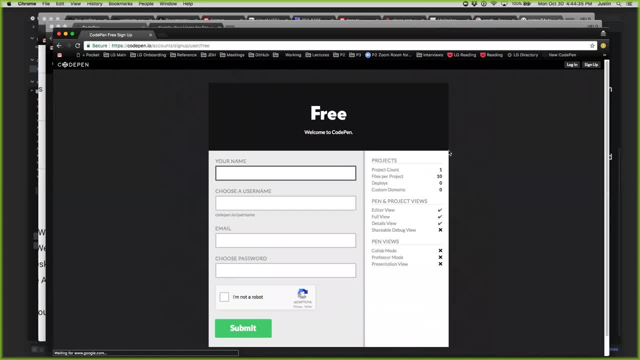 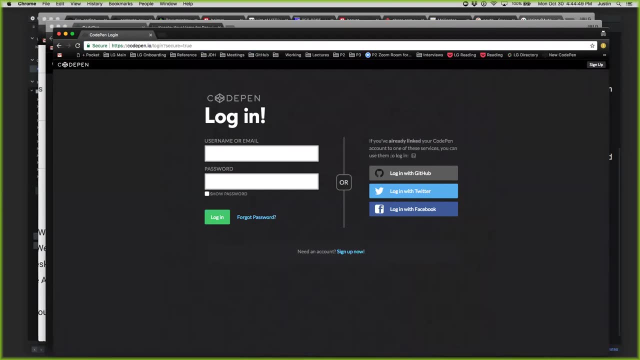 code pen in a private browser. sign up: join code pen free. huh, looks like they join code pen free. huh, looks like they join code pen free- huh, looks like they don't allow them. maybe, yeah, yeah, so I don't allow them. maybe, yeah, yeah, so I don't allow them. maybe, yeah, yeah, so I think probably. 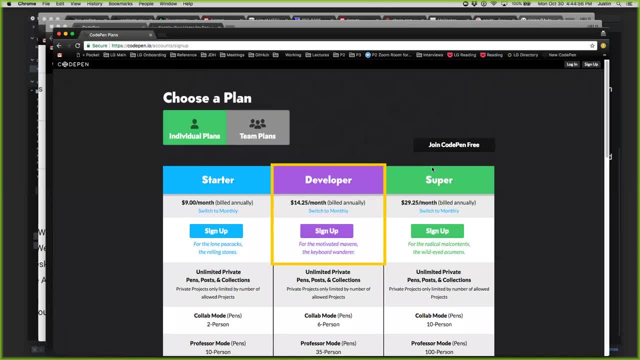 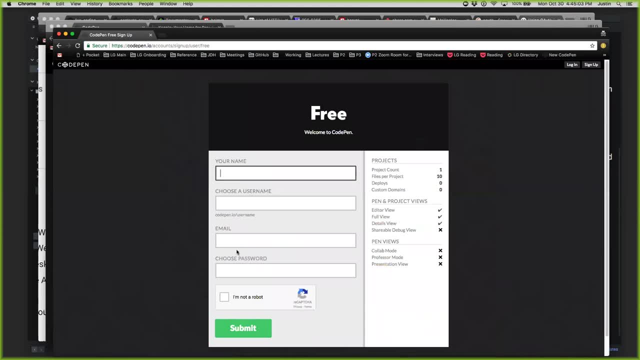 the way they do it, just judging from this, is that they have you, they have you do both. basically, they have you. pick a name, username, email and password and log in, but then you can associate a github account or a Google account or a Facebook account or whatever with your account and then, from then on, you can. 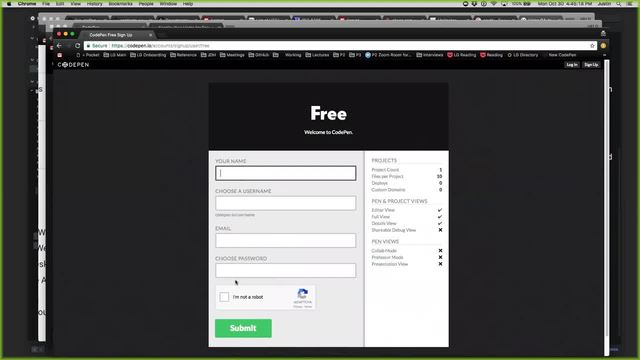 sign in. I can't quite fathom why you would do it that way. like you, you could, yeah, yeah. so I don't know why. I don't know why you would implement OAuth for future logins but not for the initial signup, because you know, with an. 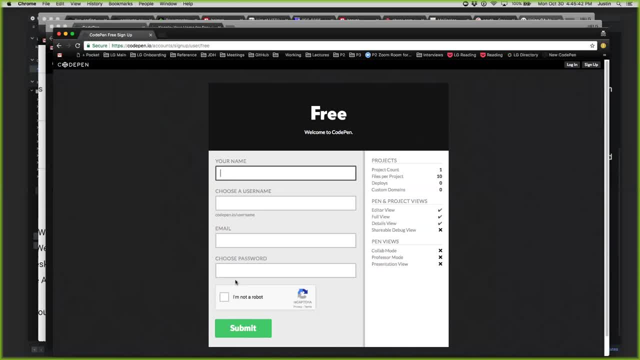 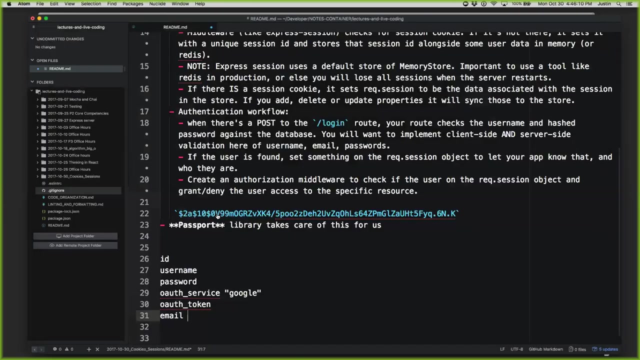 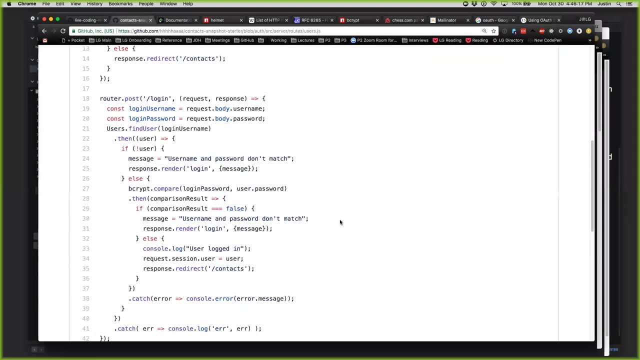 initial signup, there's nothing stopping you from also directly asking the person for information, like before we complete your signup. you need to give us this information, this information, this information. sure, yeah, yeah, it could be so. Eugene's question was about what? what is passport actually doing for us, and I'm trying to find the place. 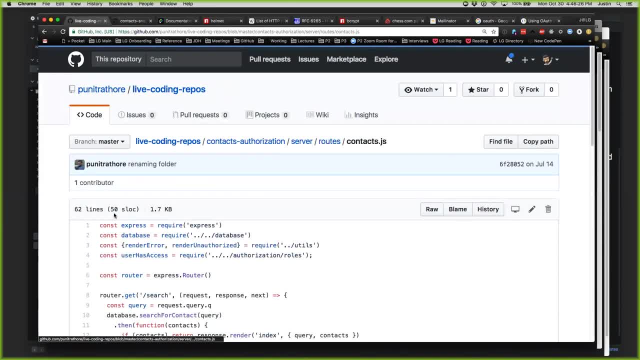 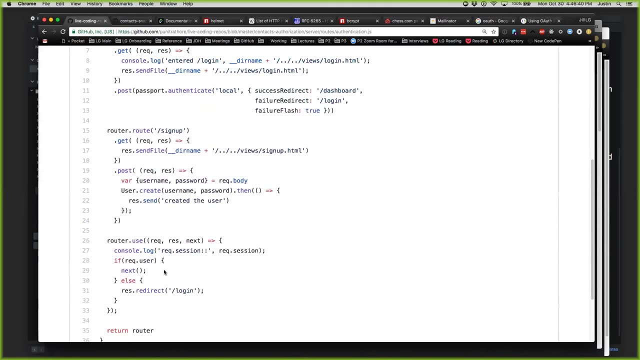 in this code where so you have to define the strategy and then how to serialize and deserialize the user. has anybody worked with passport to do that passport local? you should like. this is just sort of a general recommendation, but like build it into one of your next, one of your next projects, because 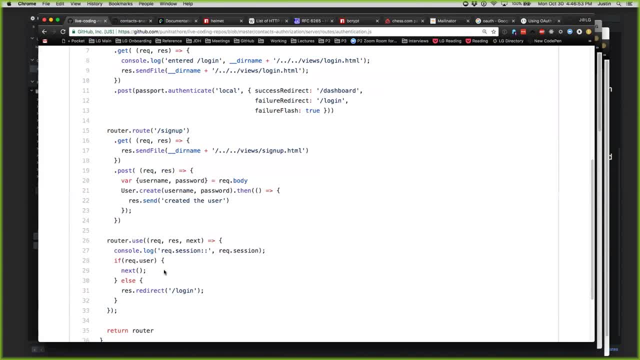 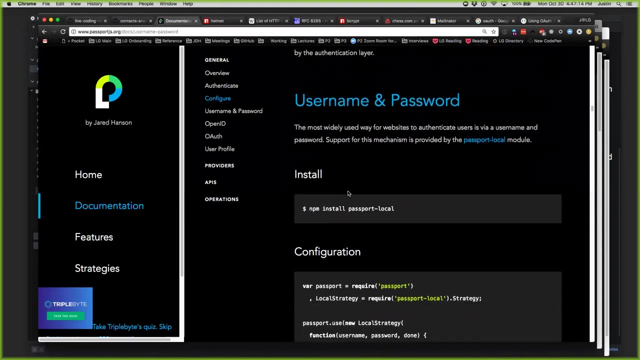 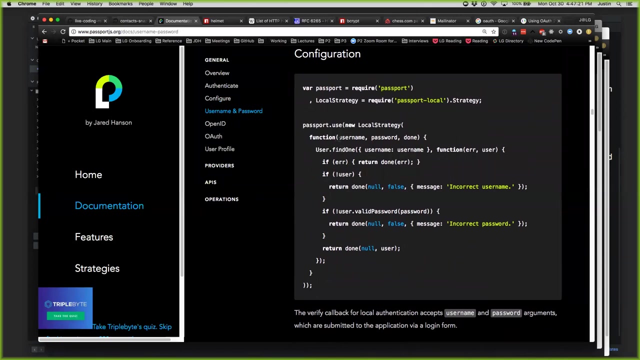 passport is like the de facto library for authentication in node and Express and it works pretty well. but it's also good to know, because it's a little bit quirky, the way it's implemented. so passport: see, I got it right. so here, yeah. so to get to, 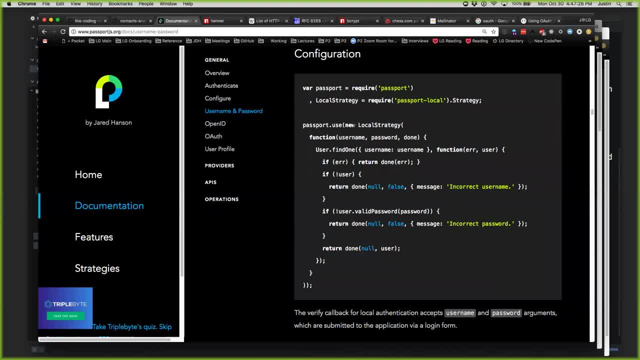 To get it working, and this is with the local strategy again. so this is: you want to do a username and password on your own system. You define a local strategy that gets the username and password and then calls the callback with in any number of cases, so you can call the callback with an error or if the user 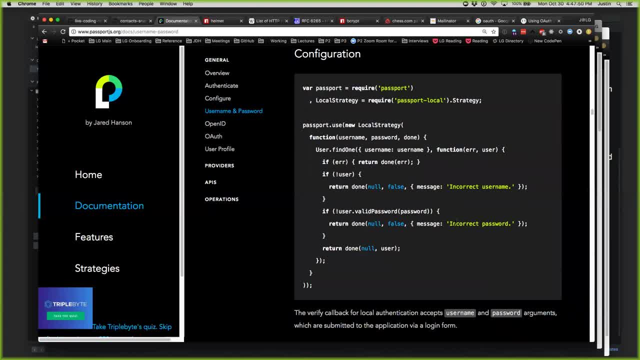 is not present, password's not correct. You know that you should never tell a user whether they messed up the username or password. You should just tell them that something was wrong. The reason is because it gives people who are trying to crack into a system a bit of 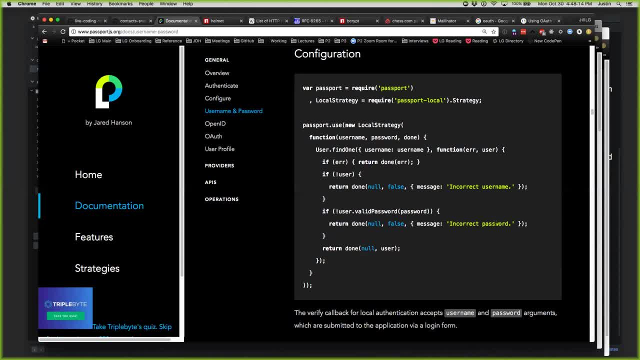 an edge If they type in some random user like, say, you were trying to hack into Brad Pitt's Apple ID account And you were like trying a bunch of usernames, and then you tried like Brad Pitt and then his birthdate or something like that, and entered a password and it said, oh, I'm sorry. 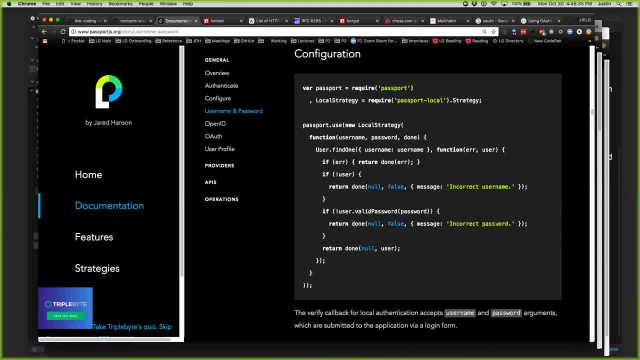 invalid password. You'd be like: oh, I know that this is a username, This is like a username in your system, because you're not telling me invalid login, you're telling me invalid password, right? Strange use case. I don't know if any of us will ever be doing that, but it does create, like this, extra 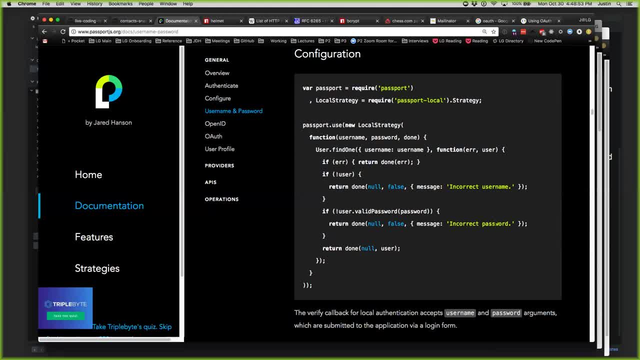 layer of security Where it's and there's no real benefit to telling someone that, like they got their username wrong or their password wrong, like- and there are usually ways to kind of address that any way, Like I forgot my password. 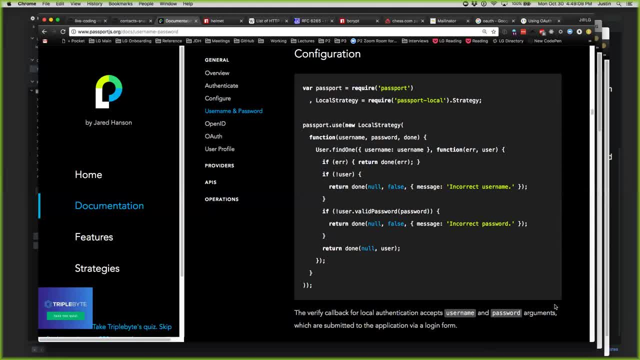 Click here. So, and why do they have to do that? So this is what's called a flash message. Has anybody implemented those? Yeah, So it was part of Express up until version three, and then they broke it out, and so 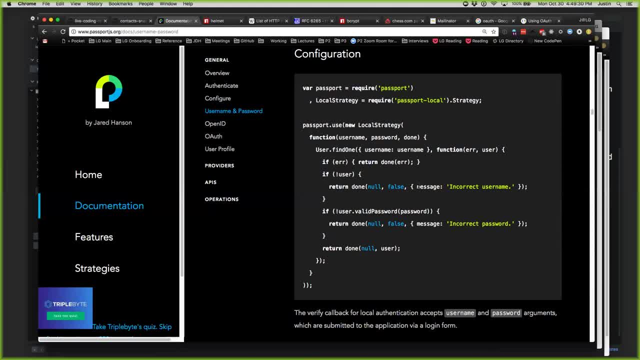 now you can have a library to plug it back in, but it's just a way of like sending a message to your front end and so that the idea of this message is that it ultimately ends up on the front end user interface saying like in red: invalid username or invalid. 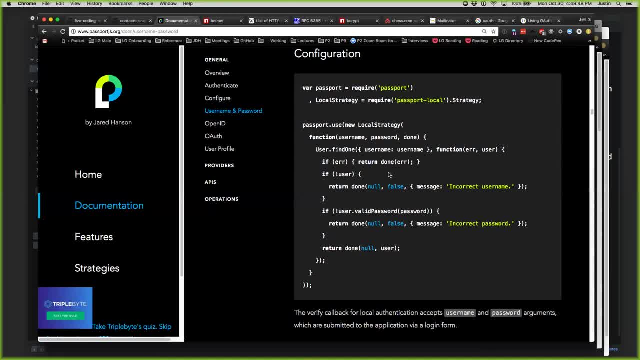 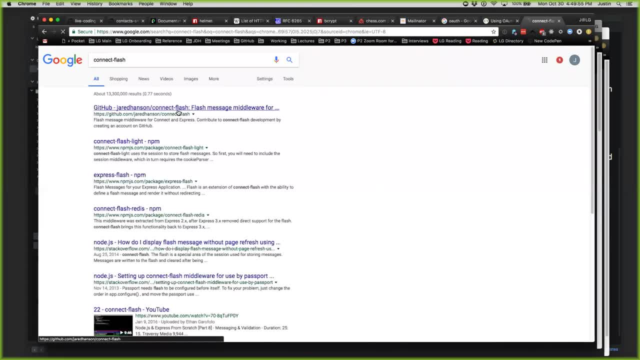 password. Yeah, I think it's called. Yeah, I think it's called. Yeah, I think it's called. Hello everyone, Hello, Hello, Hello, Hello, Hello, Hello, Hello, Yeah, So connect flash. 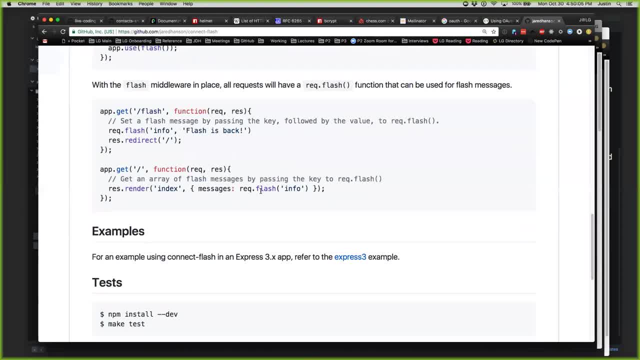 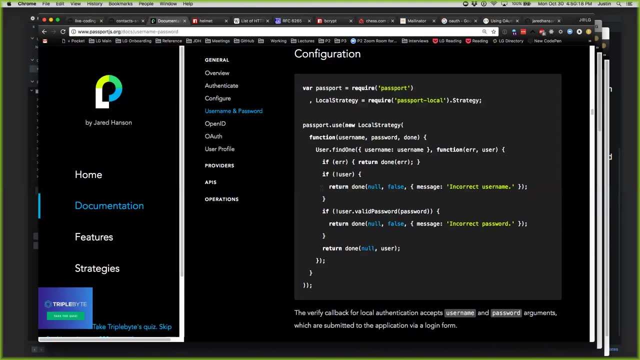 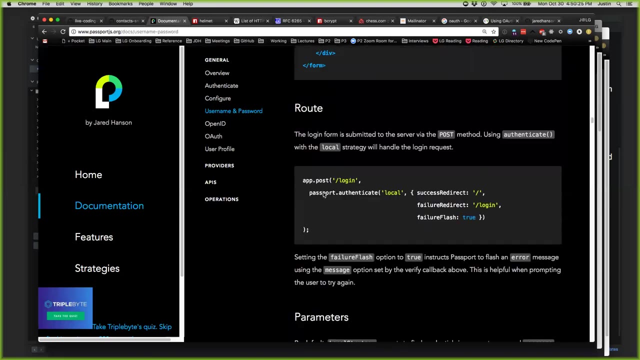 And What was that? Yeah right, Yeah, So, Yeah, So, Yeah, Yeah. So this local strategy function is kind of the heart of it, and then I wonder if it's gonna show us the serialize and deserialize Serialize. 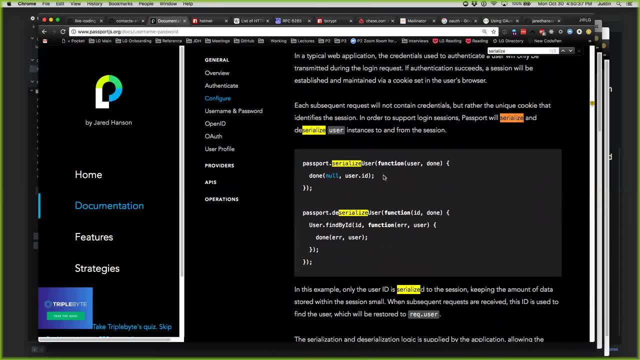 Yeah, so these are functions to. as I understand it, you wanna pass so in the serialize user. you wanna pass it, the bit of information that you want to be part of the session and then deserialize. you wanna take that out and call the done function with whatever user object. 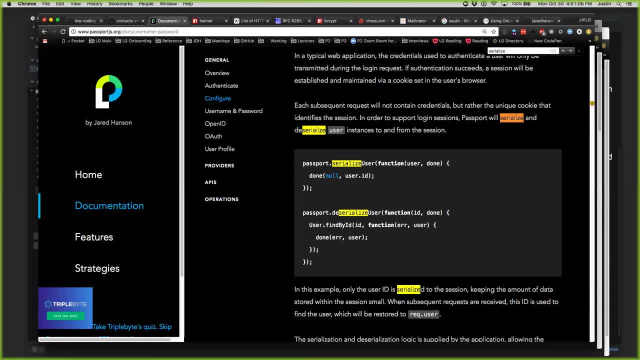 you have. so in this case they're going to a user, to their database, looking for a user finding them by ID. If they find them, then they're sending that entire user object. so that's gonna include their email and preferences. 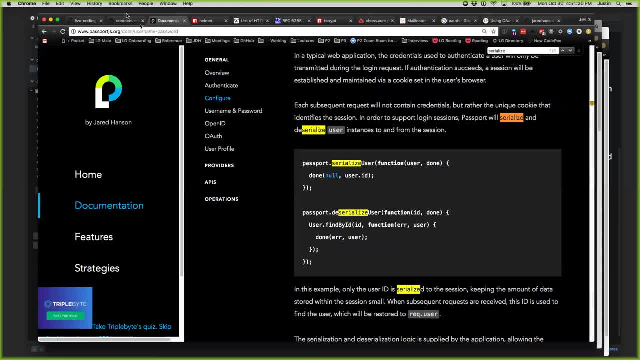 And all of that stuff Which basically takes care of most of what we were looking at before. So it strikes me as a really like one of the handful of really useful exercises to implement authentication without Passport once, so that you get the flow. 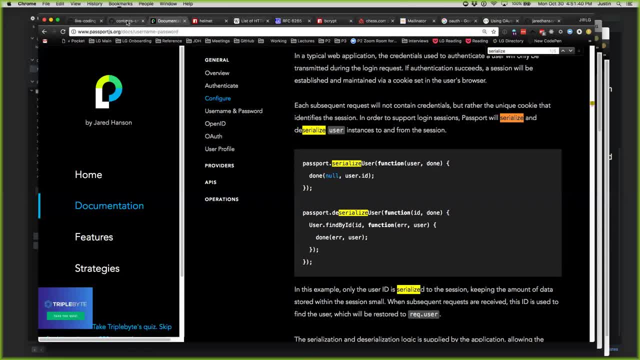 you get what's happening, you get how sessions are interacting with cookies or interacting with a database, but then using Passport way to go from there. I think that's basically all I had. You know you can do in Express. you can add things on a route-by-route basis. You can add middleware on a route-by-route. 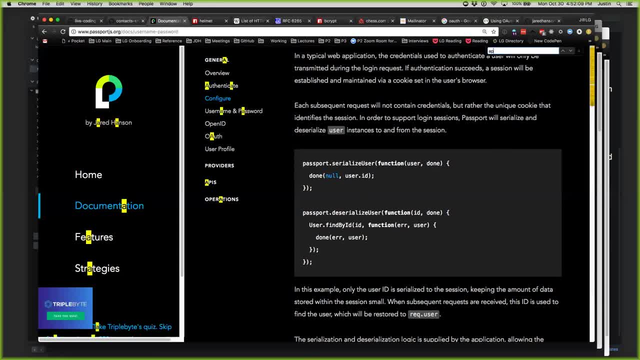 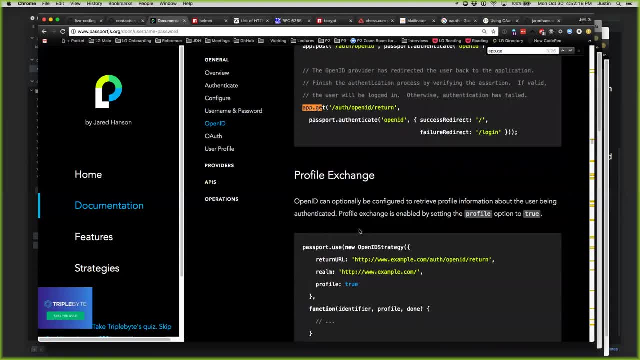 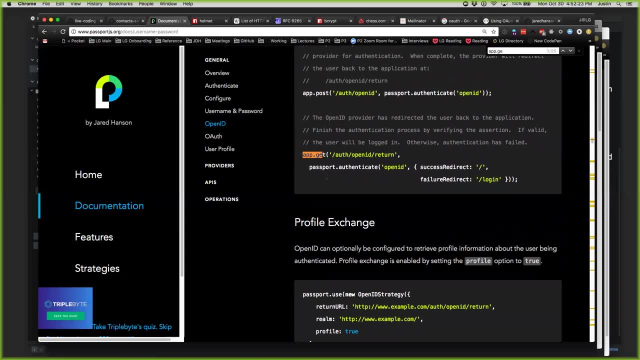 basis. So I wonder: if it's going to Yeah, so it's Yeah, so this is a middleware. Well, this is not even a middleware. This is like a route handler, I mean in Express. there's not a stark difference between the two. 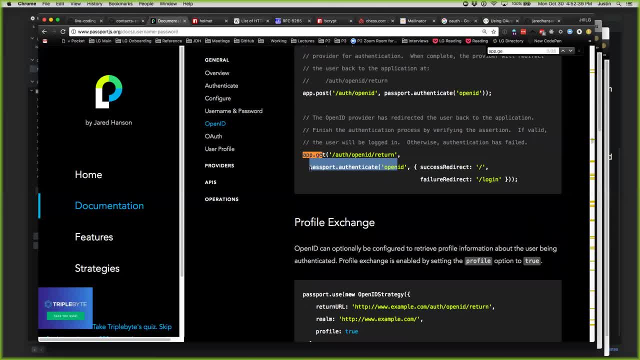 Express treats everything kind of like middleware, But what this is actually doing is Passport Authenticate is, in this case, using the OpenID strategy, But this could just as easily say local And this is the route, And if there's success it redirects there If there's a 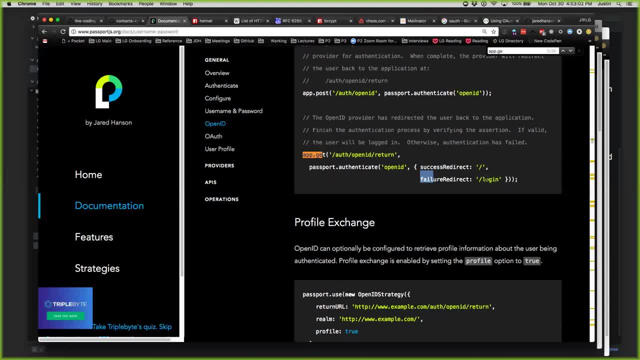 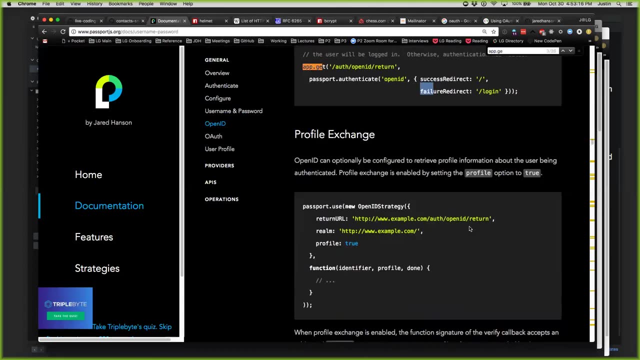 failure, it redirects back to login. So it's an entire route handler that knows to To authenticate the person And if it doesn't work, you know, if you don't successfully authenticate, then to redirect. I could talk about this all day, but I'm looking at people's faces and it's kind of like 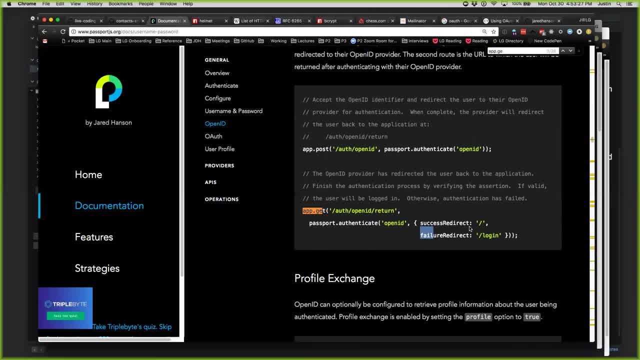 So any final questions? Has this been helpful? What's I just want to hear from a couple of people? What are you taking away from this? I don't know what the problem is. Yeah, I mean, I said Yep, Delegated Authentication. 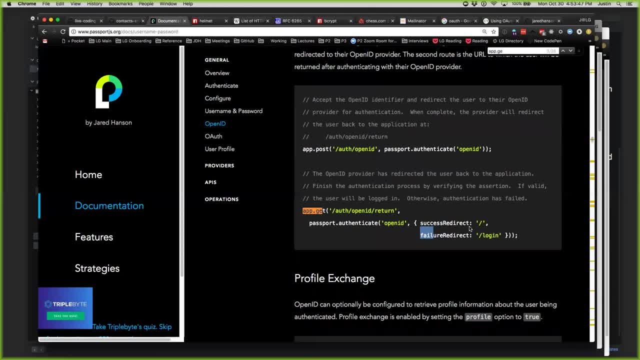 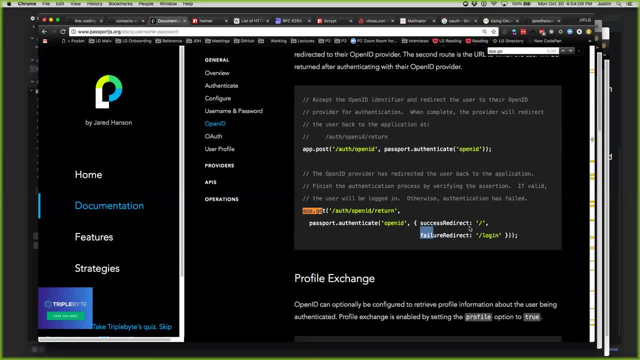 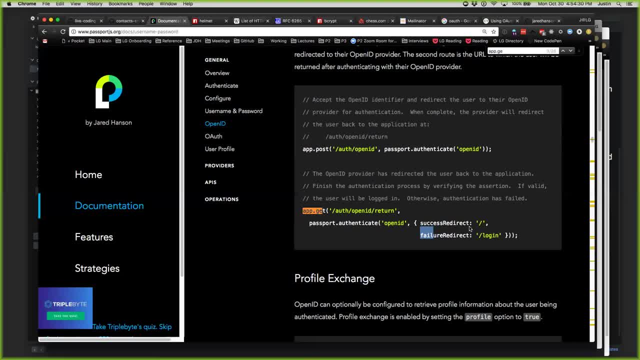 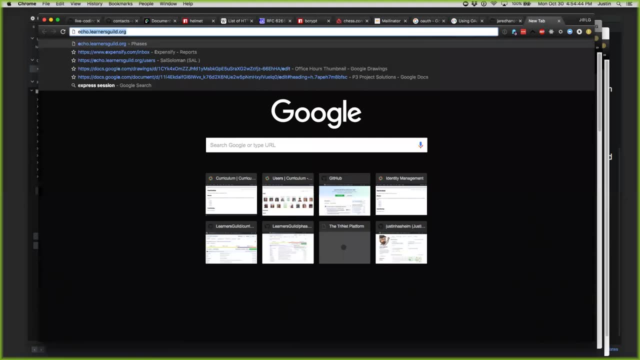 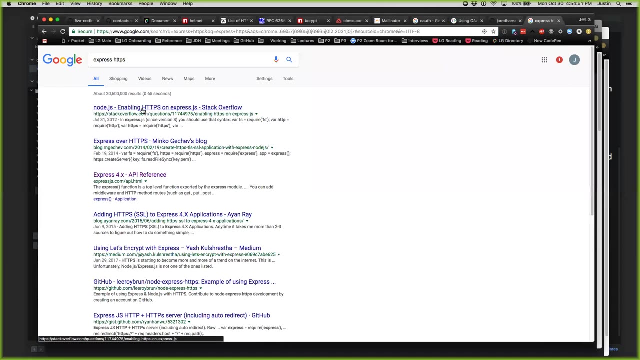 Do it. My portfolio is actually like the way you do it And then I do that as well. Yeah, or whatever. you give it the SSL and it just redirects from like that domain name to like your known password as you get the SSL. 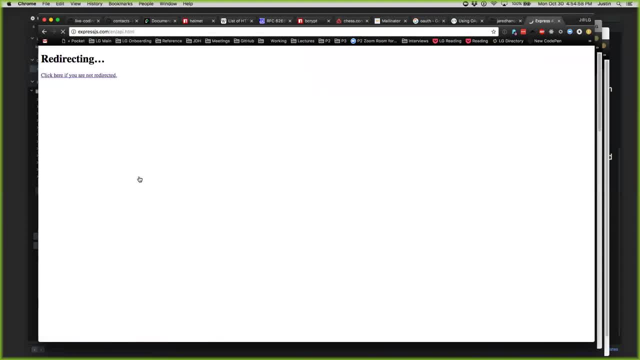 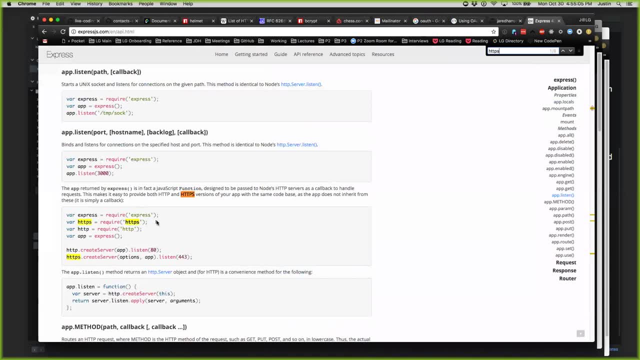 There's a website and you just download the script and then relax, And so that's with NGINX, but not Express, Right, Right, Yeah. So in any case, you're going to need a certificate, because that's the current, largely broken system that we use to authenticate the servers. 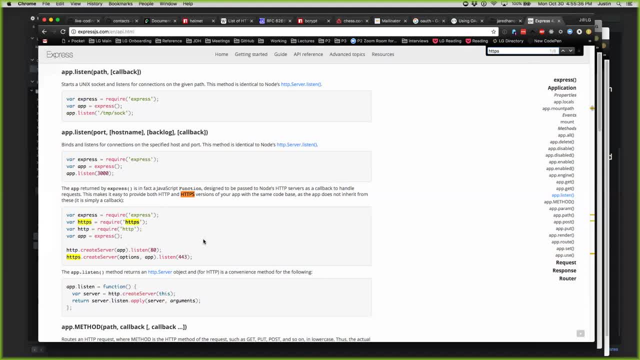 Like we've been talking about authentication. We're not authenticating clients, But these certificates are the way that you currently authenticate servers, which is like there are these certificate granting authorities and you can apply for a certificate and then get one that says this certificate granting authority that we all know is trusted. 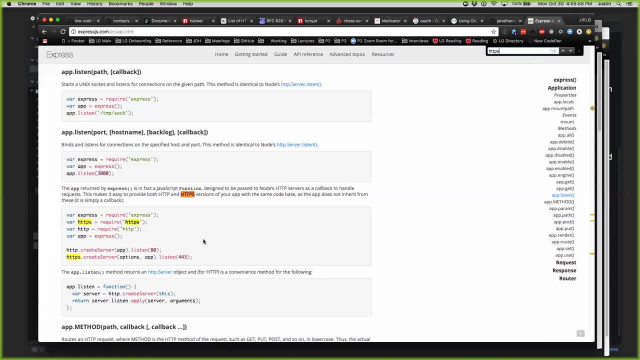 So your browser comes with like a handful of certificate authorities that it knows to trust and what their like cryptographic key is Right, And so if you see a certificate that's signed by them, you can say, okay, well, I don't know who this gen person is, but they have a certificate from. you know what's one of the big ones, whatever it is. 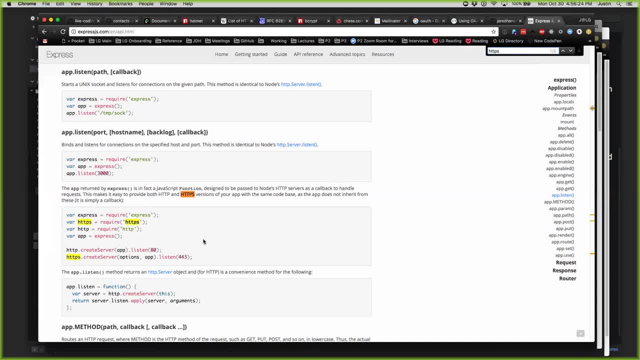 And VeriSign Right, And so we now trust this website. Let's go ahead and make a secure connection. But, interestingly, like a lot of people think that that system is pretty broken Because there's not a lot of control over who they grant certificates to. 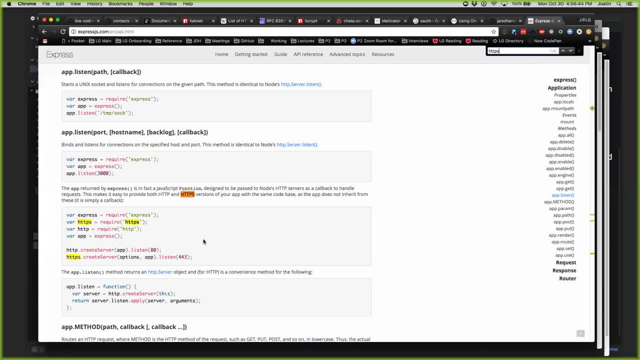 And so the degree of trust in that system is like decreasing, And one of the things that I've heard is that the blockchain actually stands to be like the solution to this, Because you can assure authenticity and trust on a much higher level, Like it's a system that's designed to create trust between two parties that don't otherwise know each other. 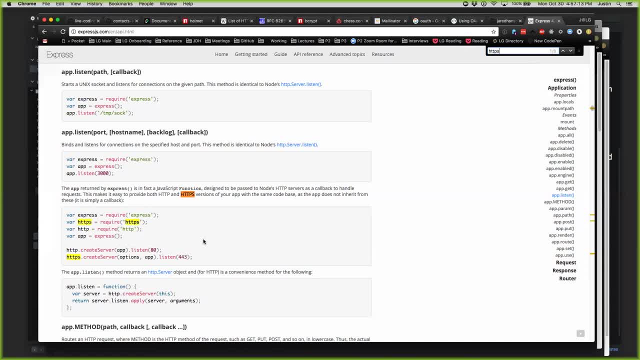 So I'd be really interested to see that system. Yeah Yeah, I don't know exactly how that would work, Because on some level it strikes me that you're still delegating Authentication to something, So OAuth is all about delegating authentication to some other service. 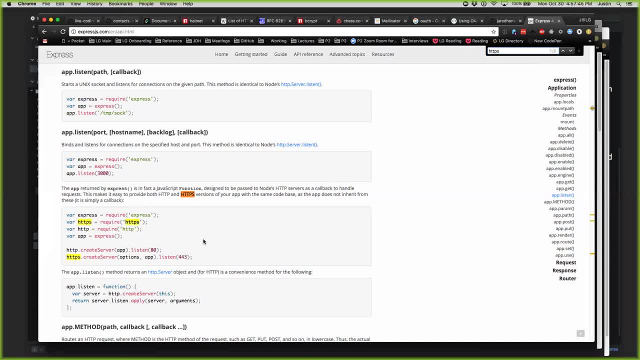 And so you'd still be sort of delegating it to like a blockchain service or blockchain server or something like that, But it would just be on the blockchain. It wouldn't have to be Google or Twitter or anybody else, Right, Yeah, But there would probably still be providers that would provide you access to that particular blockchain. 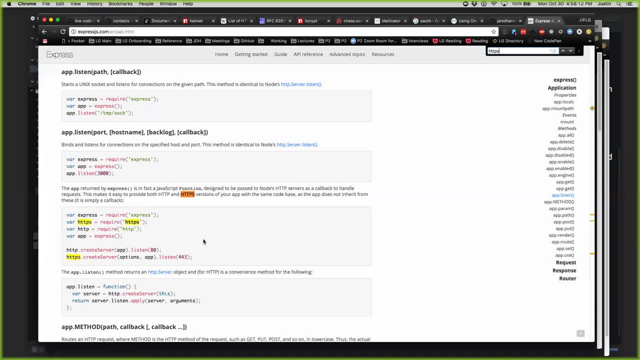 And you would probably be interfacing through them. I don't know, actually, how it would be structured, So I'd be really interested to learn. Do you pay people to do it? Yeah, So Let's say, Crypt gives you then free, fair work. 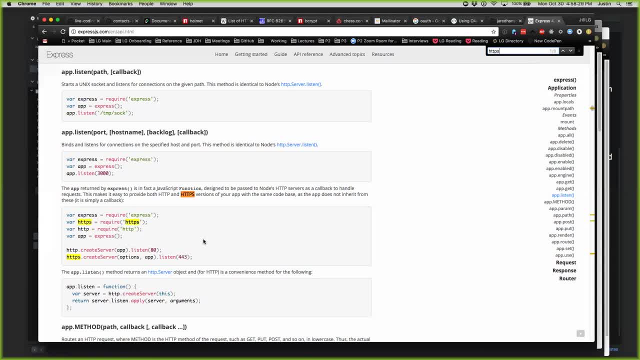 Like 30 days or something. So you can set up like a condom that'll open it up, Yeah, And then you can set it up in the middle of it, Okay, But for like a lot of higher amounts of encryption, Cool. 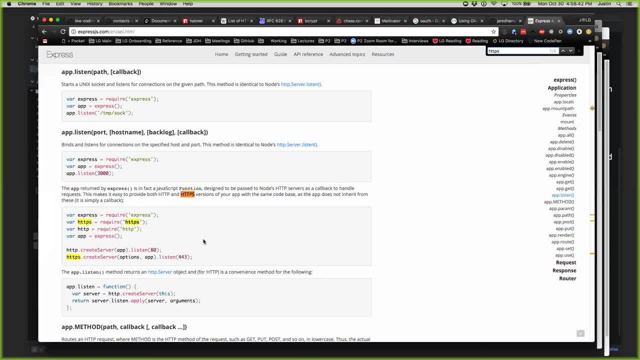